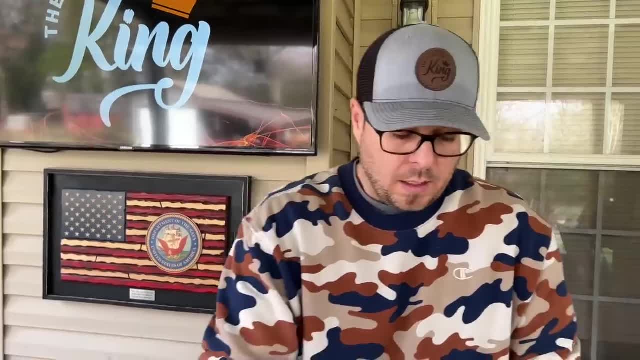 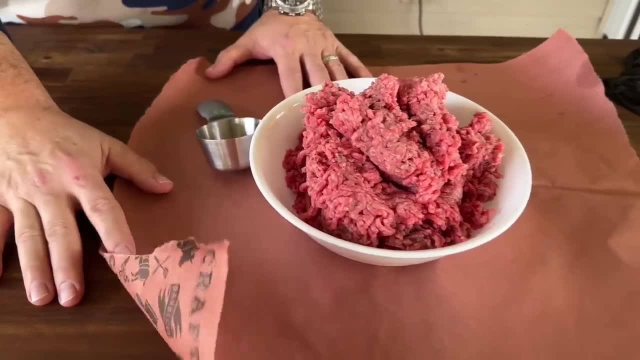 sear factor that heat. So that's what we're going to replicate right now. All right, here we go. I've got common 80-20 ground beef. okay, Little side tip, little side note, If you just got your. 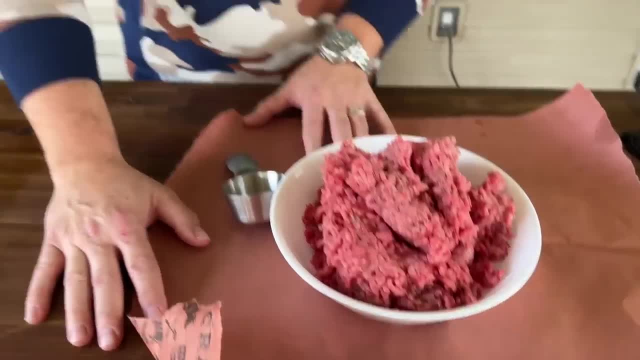 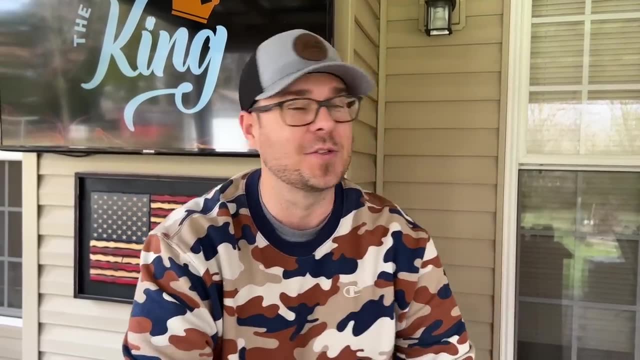 griddle and you're just starting this journey. you might not have all the tools and accessories and all the gadgets that you can have. There are a plethora. I love using that word. when it's used correctly, A standard one-third measuring cup is going to get you extremely close. 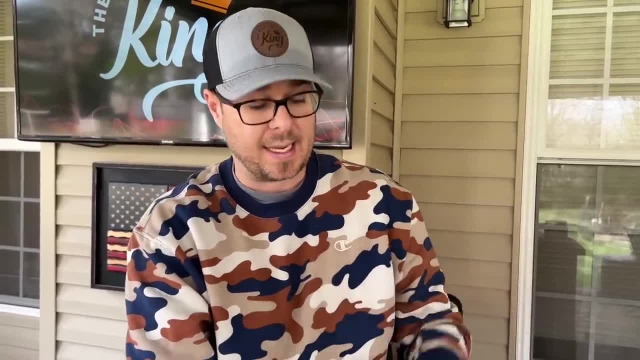 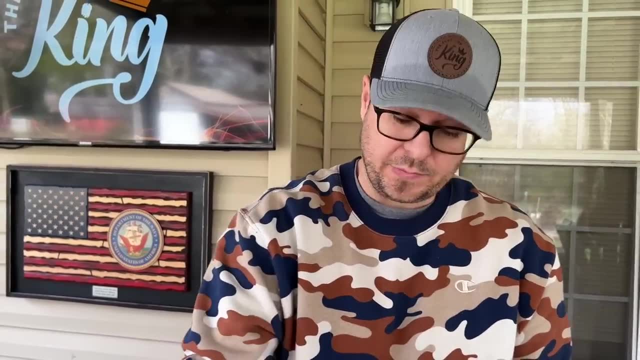 without having to worry about measuring out your ground beef balls to size. okay, So that's what we're going to do right now. How do I know if my griddle's even hot enough? That's a whole different video in itself. okay, What I'm going to try to show you if you don't have an infrared thermometer. 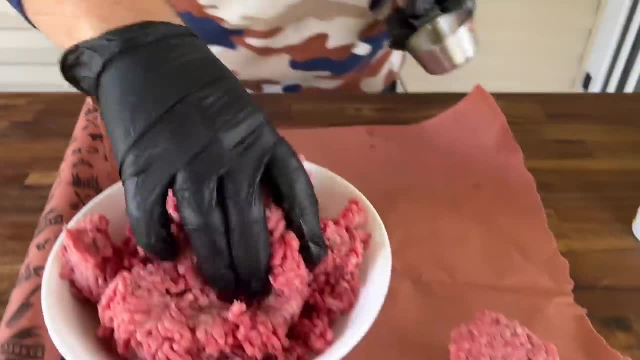 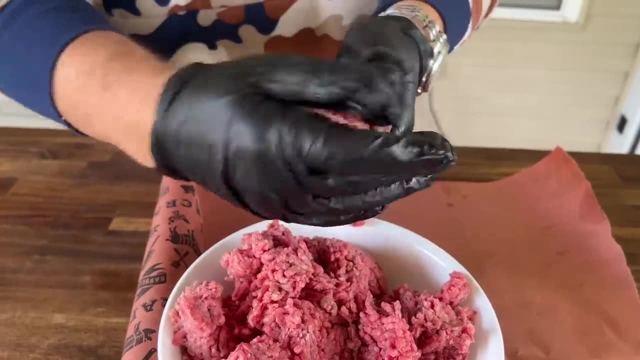 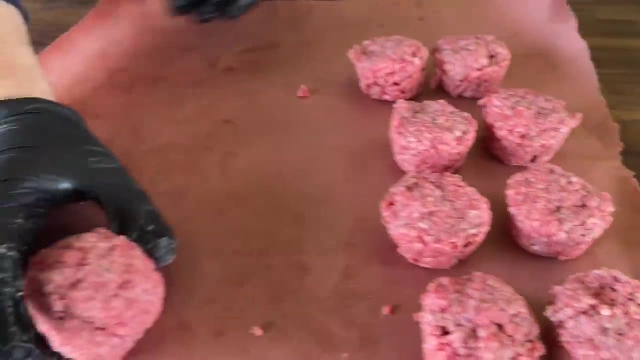 is the way your meat reacts By using common ingredients that you already have. okay, You don't have to have every single tool to the trade the very first day you get your griddle. Now that you got all your balls measured out, just ignore this one. Obviously, you can see the size of that We're going to get. 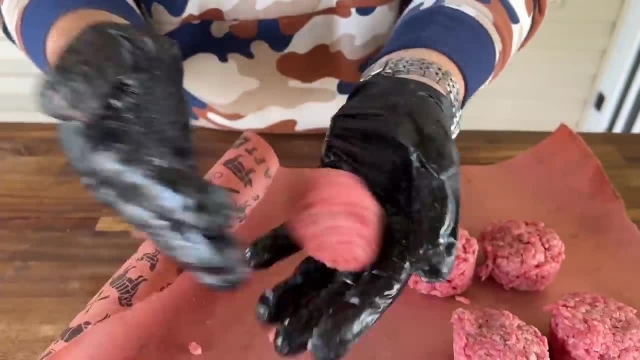 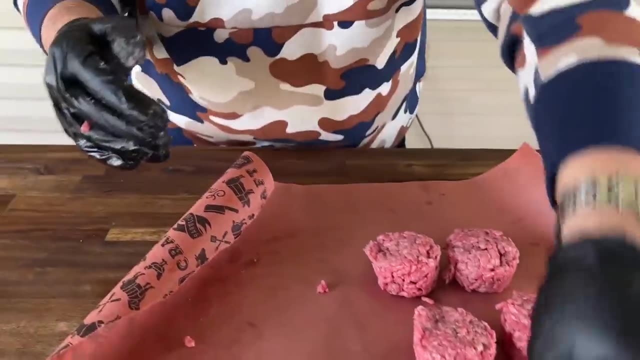 to that one later. Just try to roll them out loosely, pack, right, You don't want to overpack them too much because you want that lace effect. The harder you pack them, the tighter your beef is going to be and the more or less tender that your ground beef is going to be. 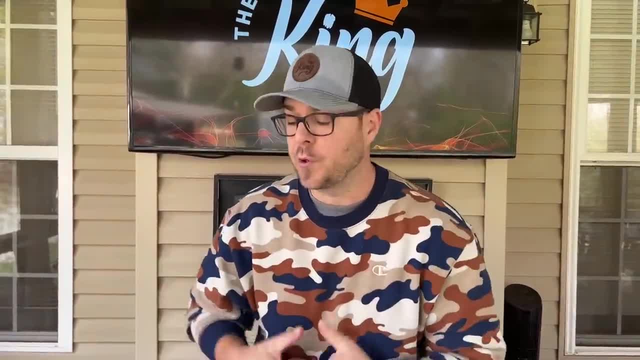 Mistake number one: your griddle's not hot enough. You're not used to it. You're not used to how much BTUs, how much force it takes to heat up your griddle, whether it be a one, two, three, four. 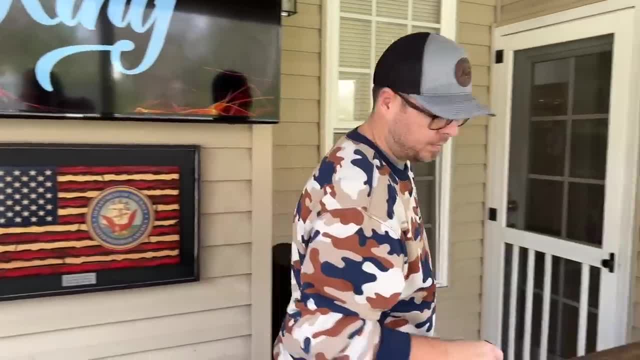 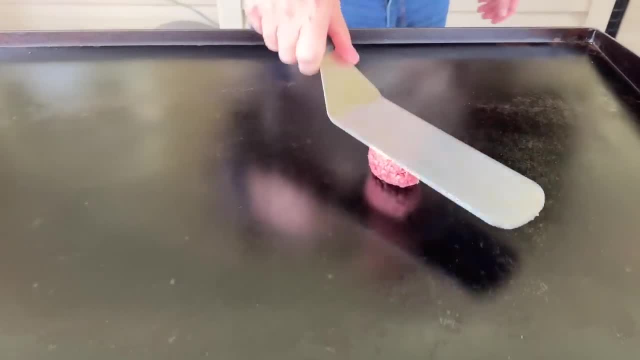 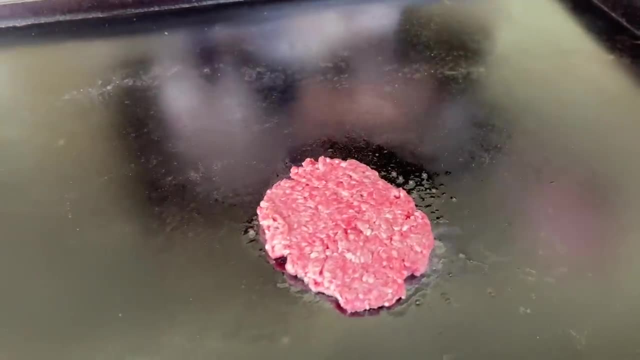 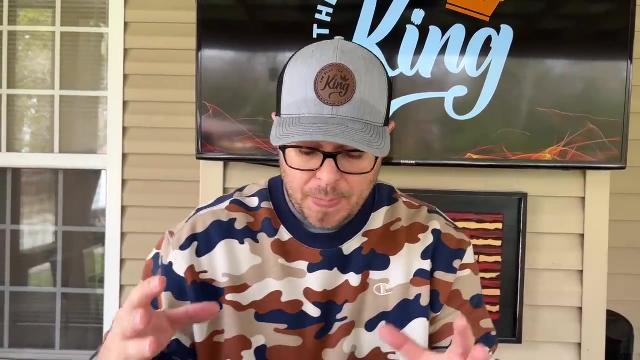 or even six burner right. So mistake number one. Mistake number one is not having your griddle hot enough. What happens is it's going to take a lot longer, and we just mentioned this. a lot of things circle each other back right. It's going to take. 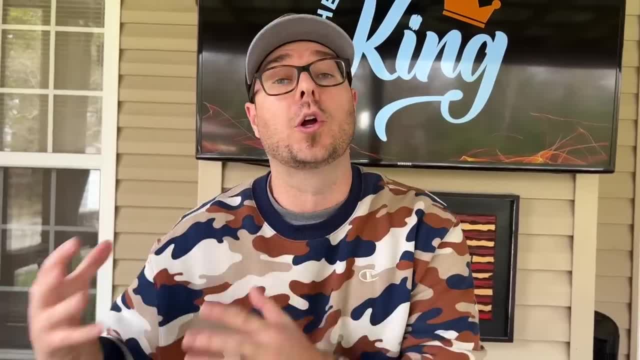 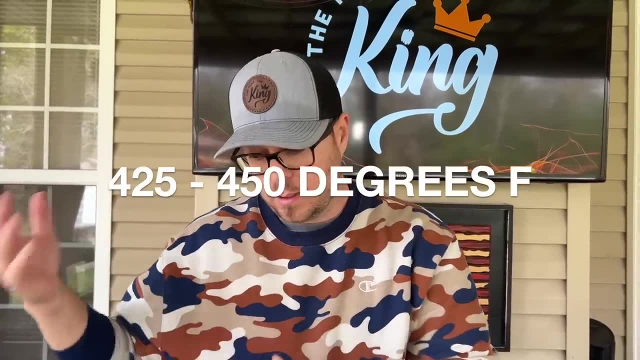 a lot longer for your crust to build. If it takes that long, then you're overcooking your burger. These burgers are fast and quick. okay, You want to make sure that your griddle is heated up or heated appropriately to handle the coldness of the burger? All right, now that your burger's cooked about 50%. 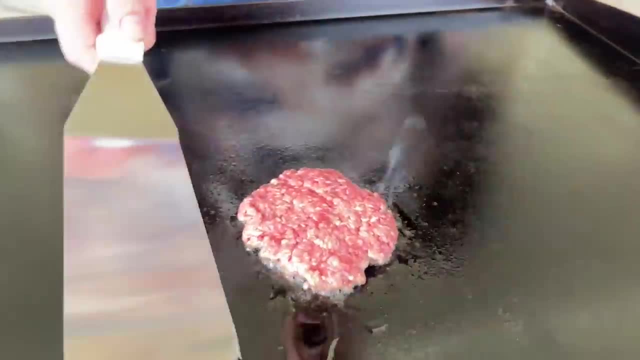 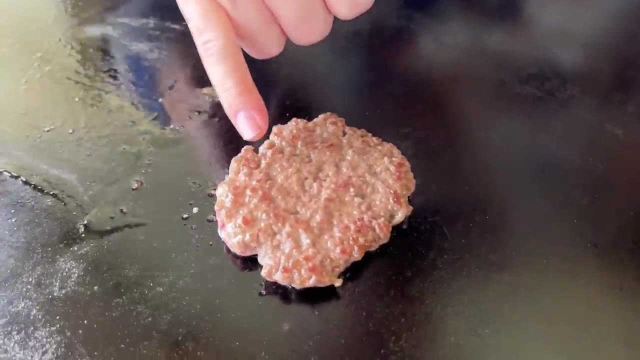 the way through, which is this traditional standard burger philosophy. we're going to flip it Now for the newbies out there. you notice how there's really no dark color Now. the burger's moist, so you guys can see it right there. That is a lot of moisture left in the burgers. When they say you 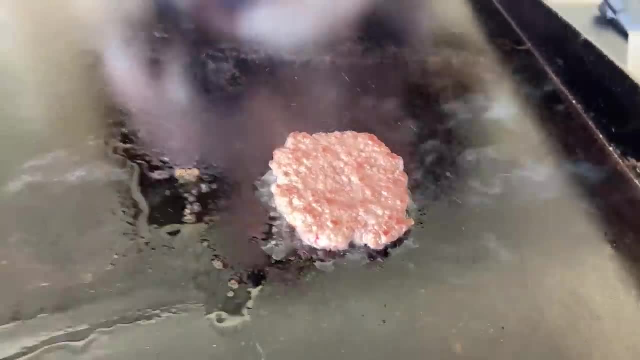 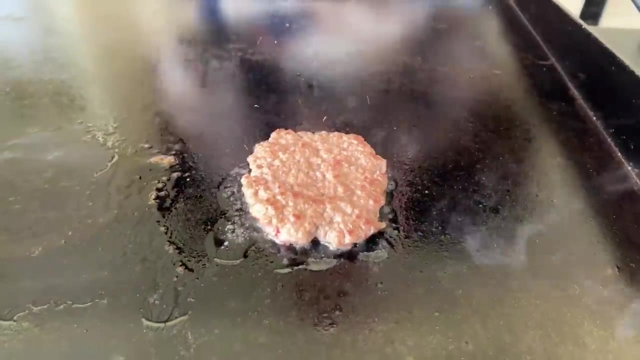 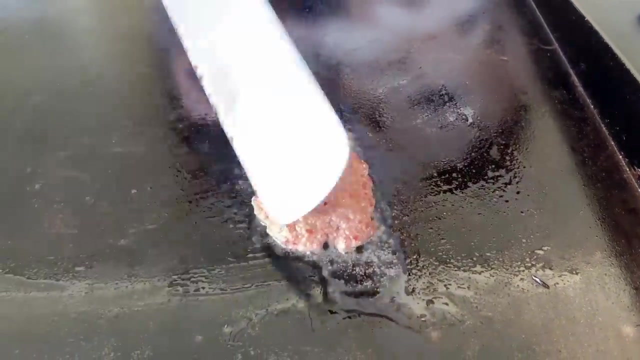 cannot get a juicy, smash burger. it's just not true. okay, All right, but there's no color, There's no Maillard reaction, and that is what everybody craves when they're talking about a burger. okay, All right. just to recap. you guys can see the difference. Keep this in your back. 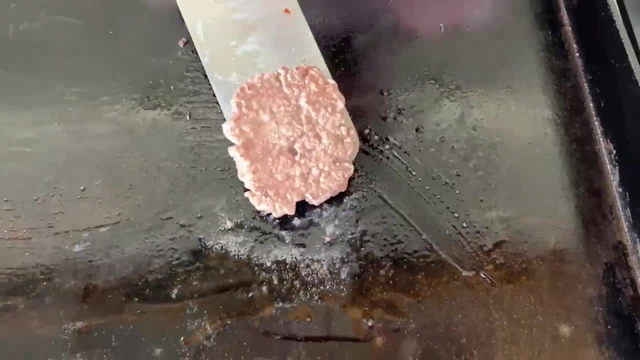 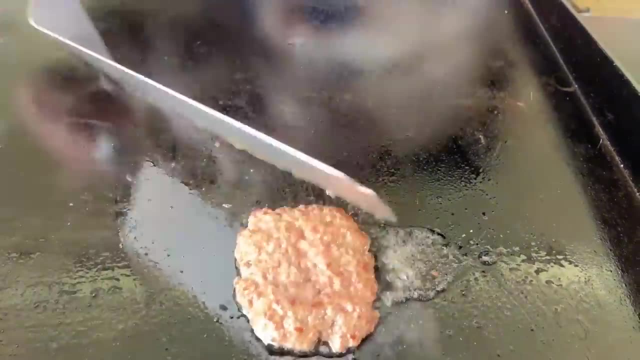 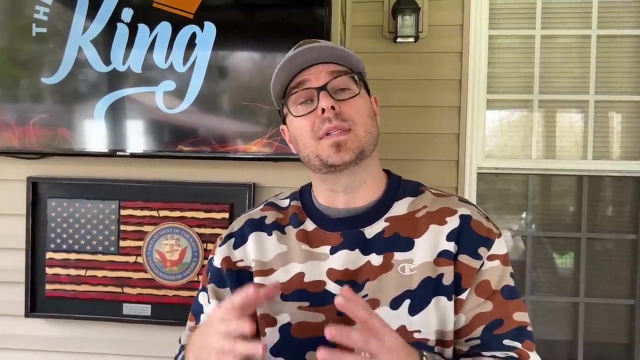 pocket what it looks like. okay, See how just grayish it is. Just keep that in mind as we keep cooking. So this is your griddle being too cold, not hot enough. Number two on the list. the proper technique is kind of like it's not a scientific technique. 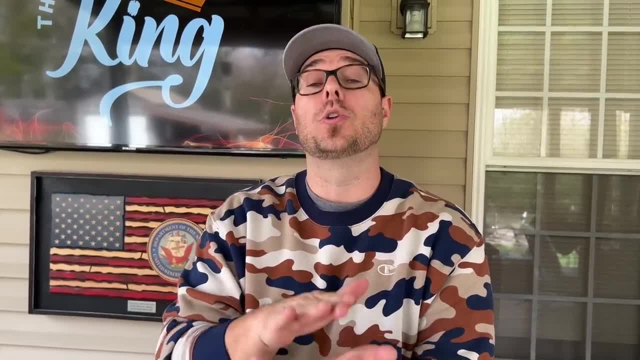 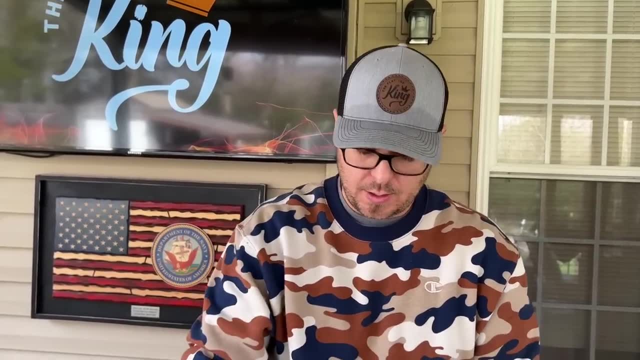 but it's definitely out there, The idea of smashing and holding your burger on the griddle, all areas to get that great contact that you need to create the Maillard reaction. okay, So what we're going to do is put on the griddle. 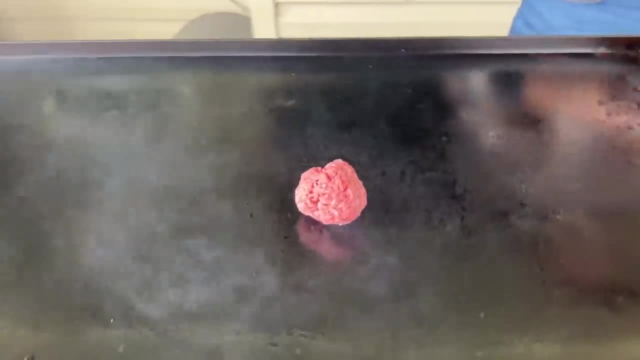 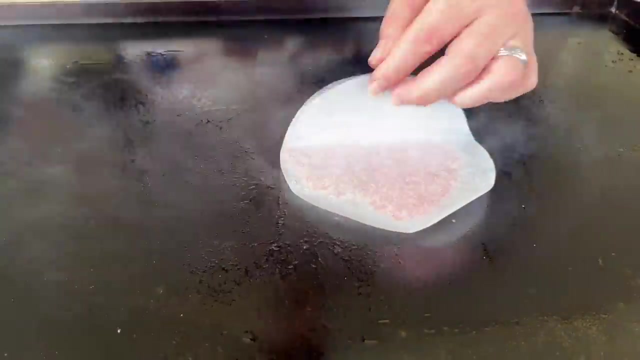 we're going to smash it and leave it right away, okay, So we are making the mistakes Absolutely On purpose. Yes, One thing too: I see a lot of people do, and you notice how we have a lip here. 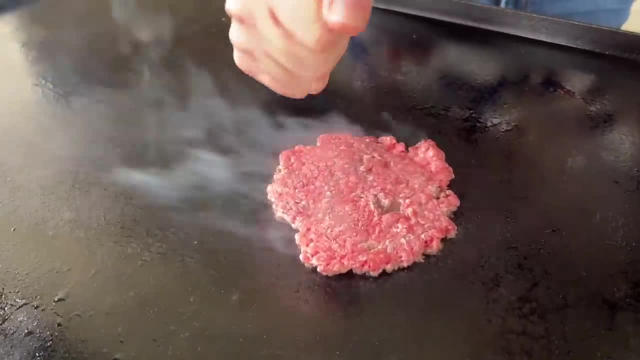 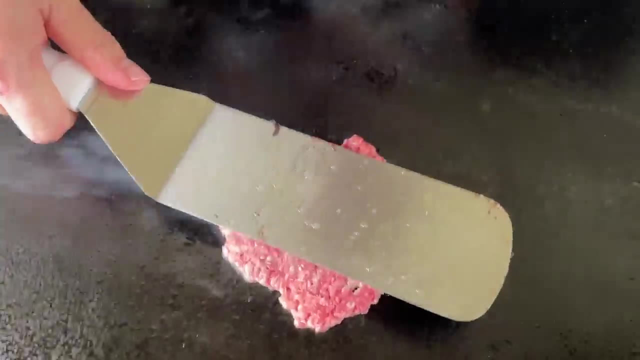 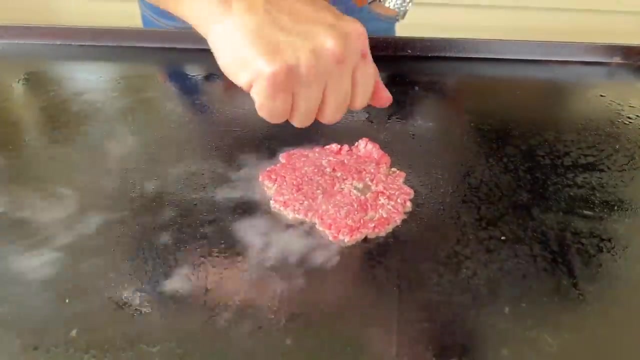 Okay, People smash it, but they're not rocking it back and forth down. When you do that, you're going to have uneven lips, depending on how wide your meat press is or your spatula. okay, So, not only is it not holding it, it's not rotating it around to make sure you have even 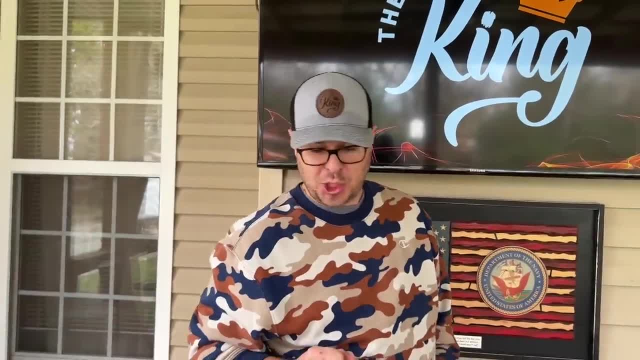 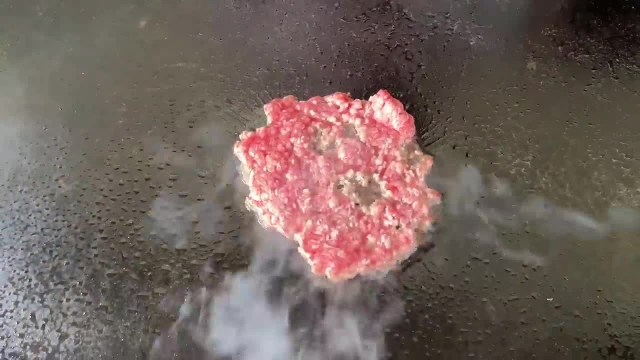 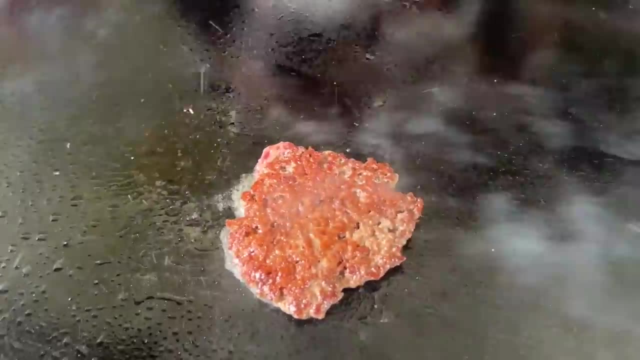 smash-age, Even Smash-age, Smash-age, That's a culinary term of the day. All right, You see how we're lacy inside. That's a telltale sign We're going to flip. See how we don't have even coverage. 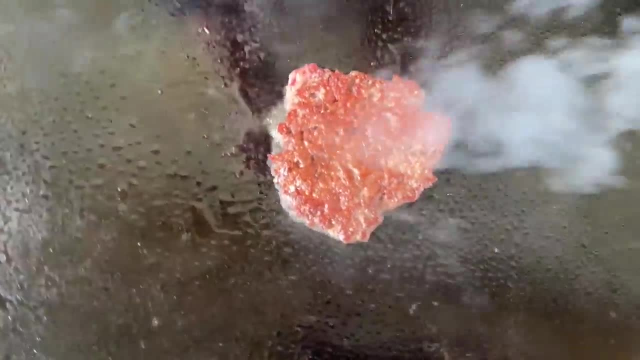 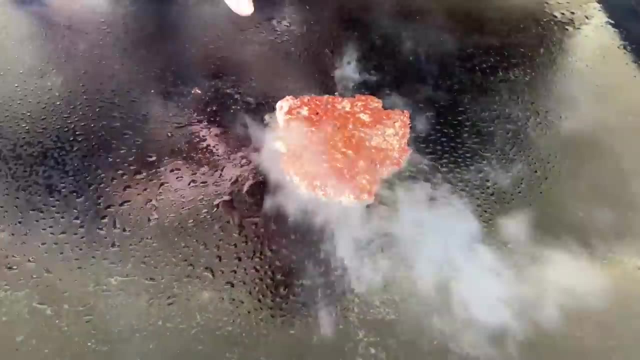 so you're so close that it could be a little bit better. right now you start seeing the darkening that we're talking about. when you're talking about smash burgers, that's one, two, since we didn't get the even smash burger to begin with. you notice how our burgers a little bit raw up here. 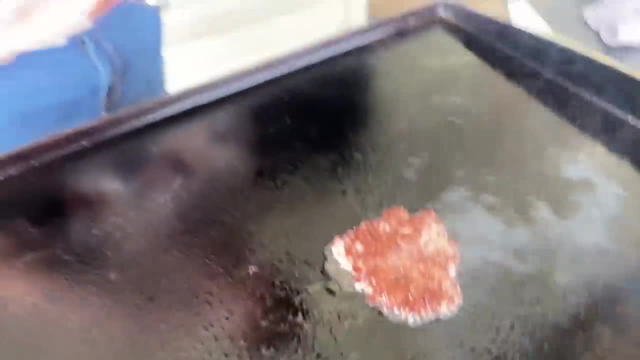 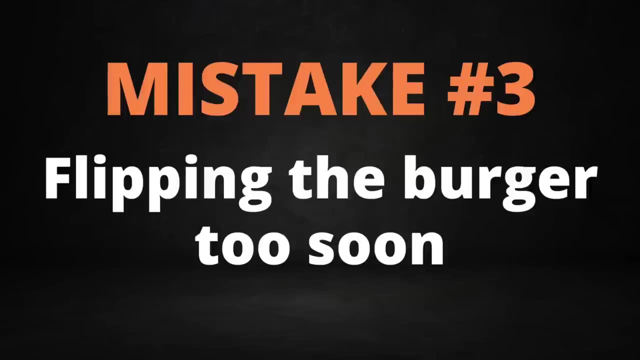 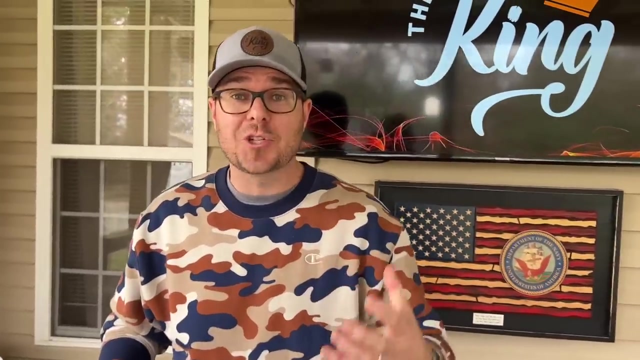 that's not necessarily a problem, but it's not perfect. when you're talking about the perfect smash burger for beginners, it's the little things that matter. number three on the list: flipping too soon, not allowing that reaction to happen. okay, you've done everything right so far. you've got your correct measurements, you've got the correct temperature. 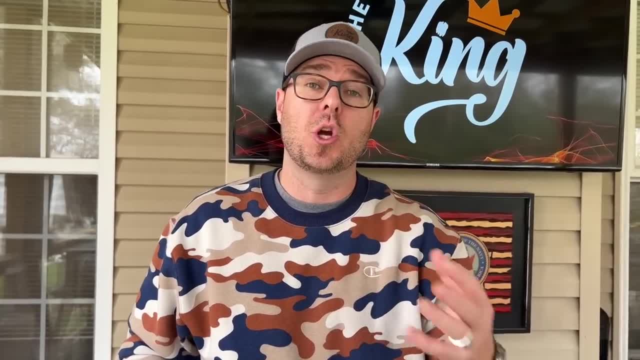 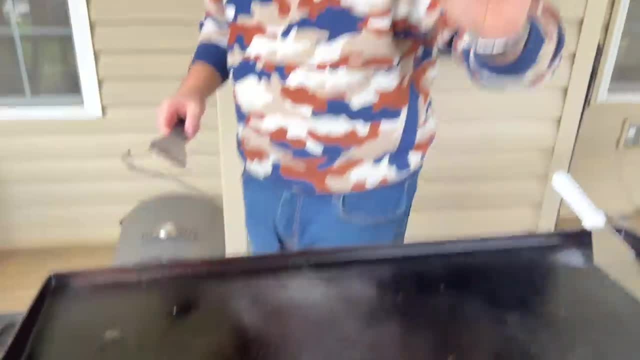 on the griddle. you're going to smash it correctly, but what if you're in a rush or you're not confident and you're scared that you're going to overcook it? okay, i'm going to have a link in the description with these, if you guys are serious about making your burgers. uh, we've had our griddle. 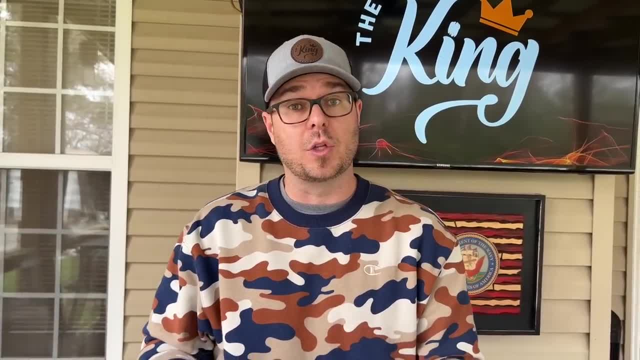 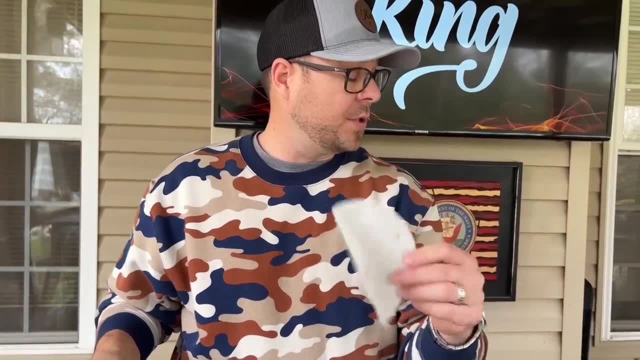 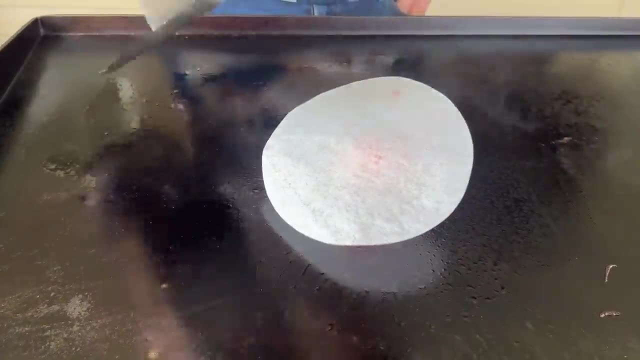 for two years and ever since then i've just used the long sheet of parchment paper and had to cut out in triangles or squares or circles myself. we found these little doohickeys online and they have been incredible. definitely takes the guesswork out of it. all right, you ready, we'll smash it the right. 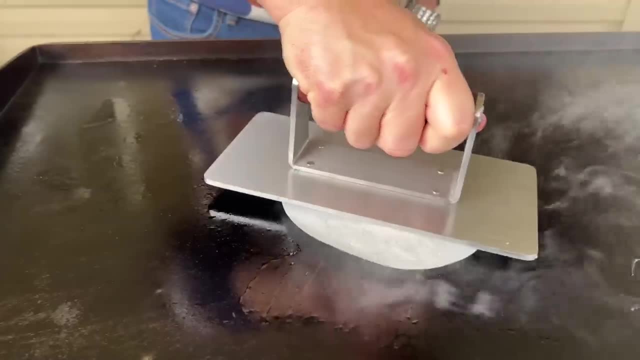 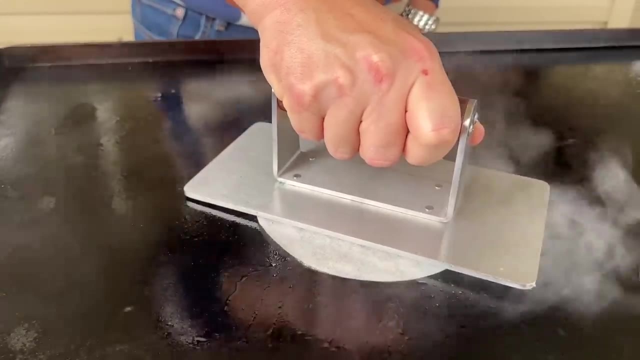 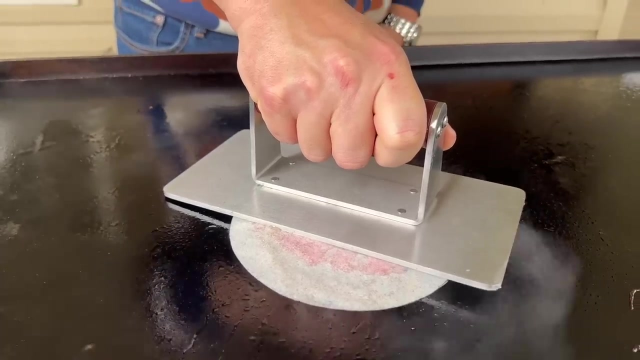 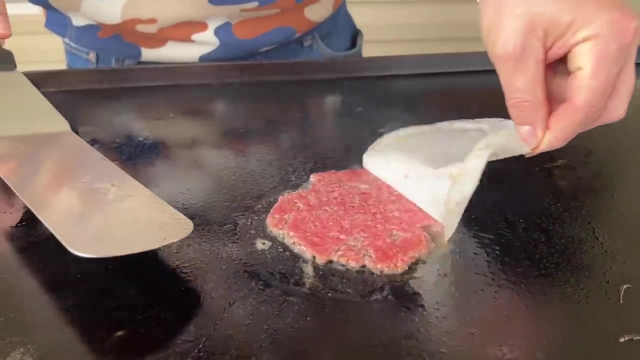 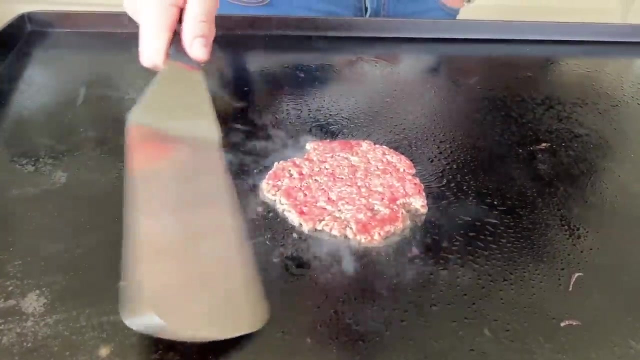 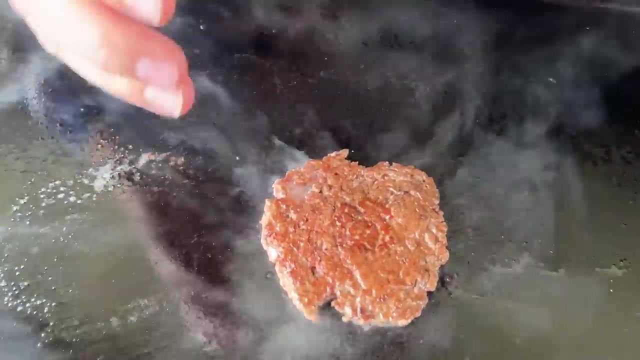 way, work around with it right even once we get it to where we like it, we're going to hold it for 10 seconds and then we're going to flip it too soon. yes, you guys ready. see the difference. see how we don't have that deep golden brown all the way across. 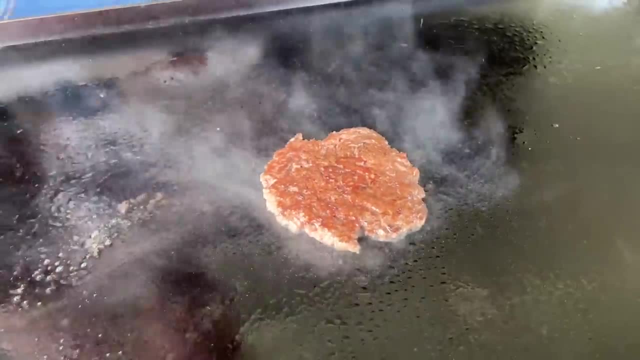 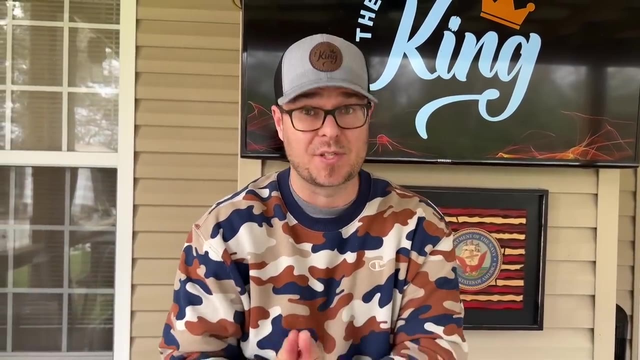 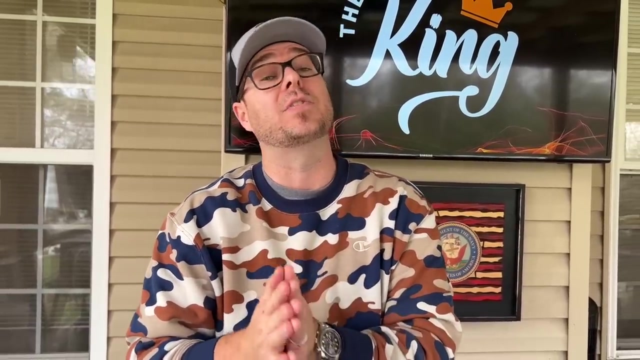 because we're too worried about letting the burger do it it's supposed to do. you've got to let the burger fry in its juices. um, that's what makes the smash burger. okay, you can have a smash burger without the maillard reaction, but once you conquer this method and taste the difference of what it makes, 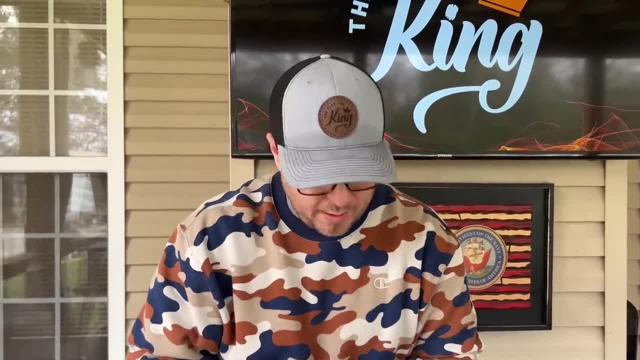 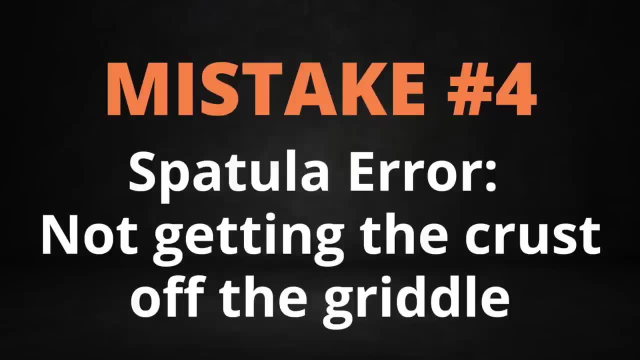 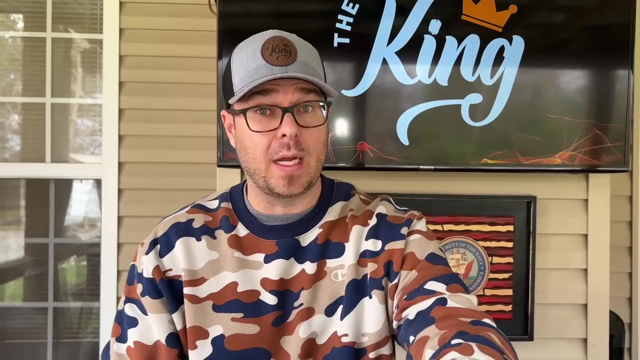 do you believe it makes a difference? yes, way to really hammer. i love smash burgers made by you, not made by me. there is a big difference. number four: the correct way could be many different ways. i'm not saying my way is the perfect way, but there is a rhyme reason to the madness. right, you have to get the crust off the. 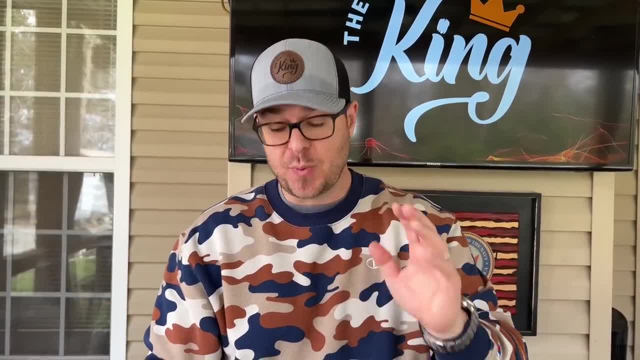 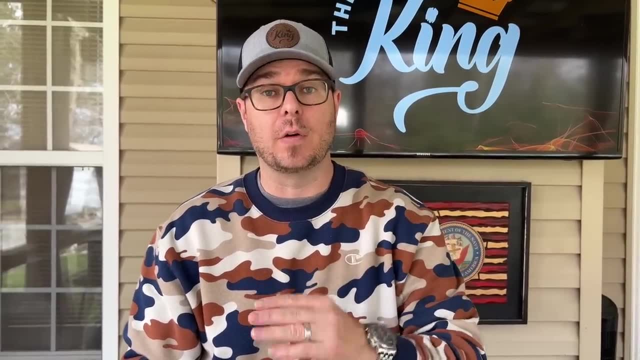 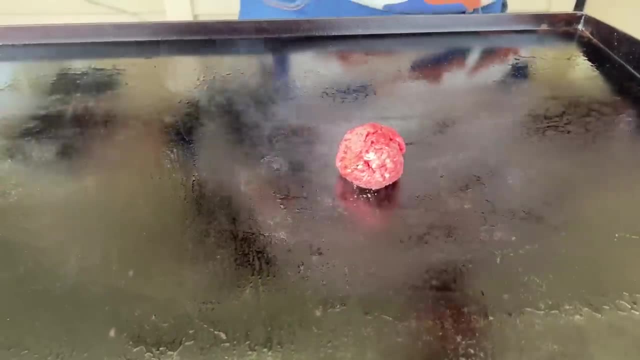 griddle. you cannot assume that just because you've done the perfect flat top seasoning, the perfect griddle seasoning, that your spatula is not going to do the job itself. you have to help it, which is why we love these spatulas. okay, press, hold 10 seconds. 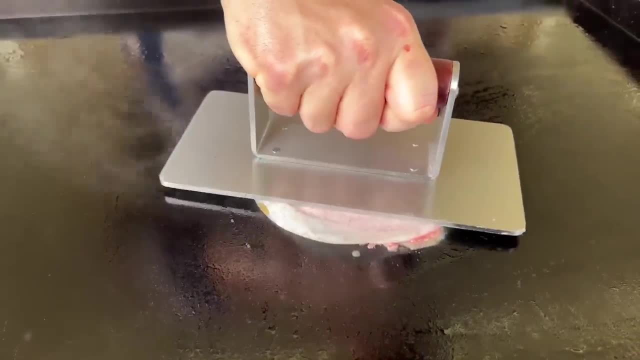 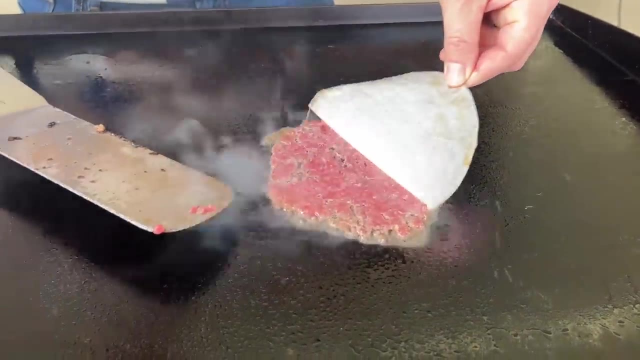 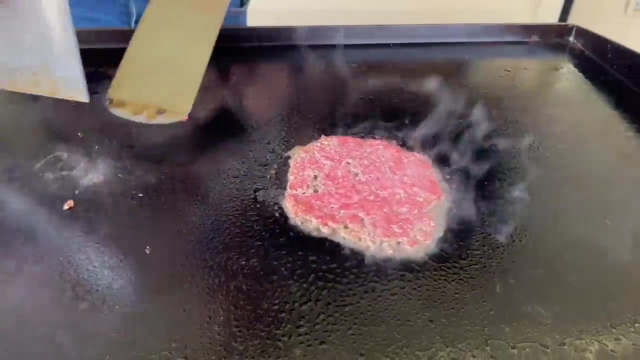 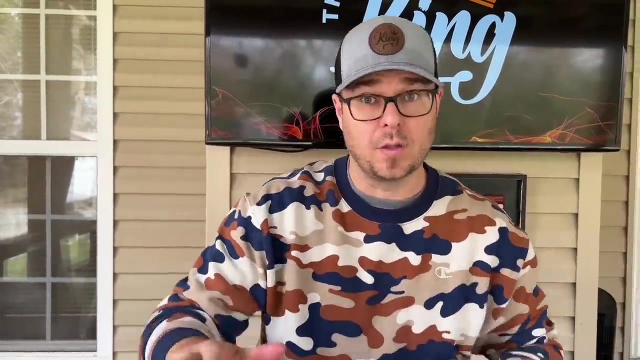 10 seconds, even press. we're doing everything right. okay, i would say right now we're shooting low 400s. okay, maybe middle 400s. these burgers do not take long to cook. we have not stopped filming and notice how we're starting to get browning. you want? 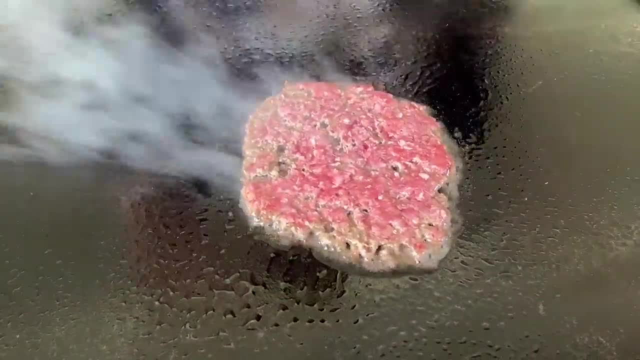 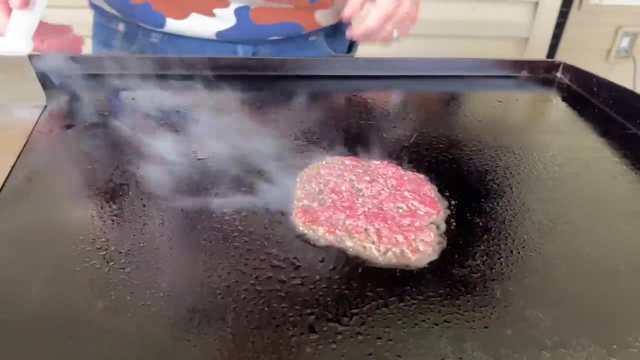 to go just a little bit longer, right, it hasn't been on the flat top that long. and this is what happens. that burger is a hair in itself to the griddle, okay, even though there's a lot of grease, it's pushing the grease out. what you want to do is come in on a side motion, okay. 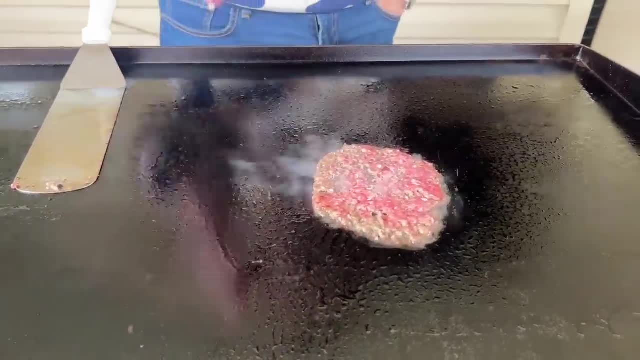 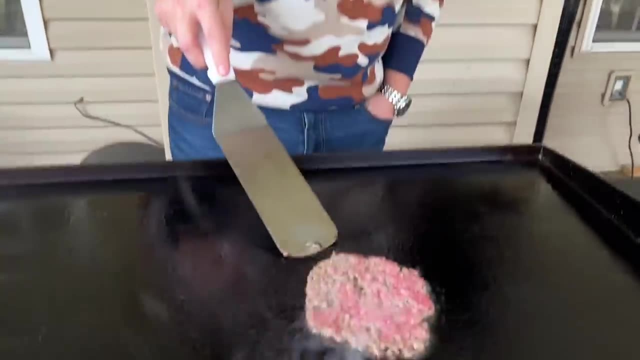 and you want to be able to get in that angle that doesn't hurt your flat top but also helps the crust off the griddle. okay, so are you going to do it wrong to show them? yes, what you don't want to do is come at it like this: 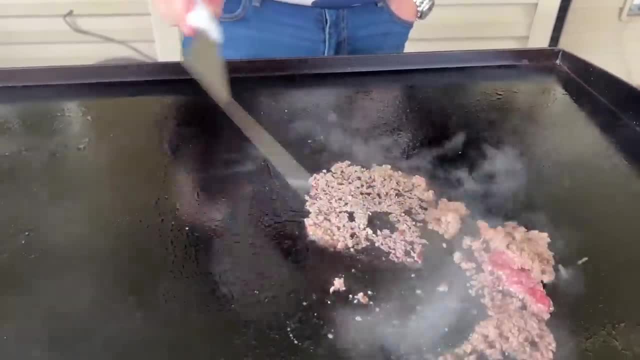 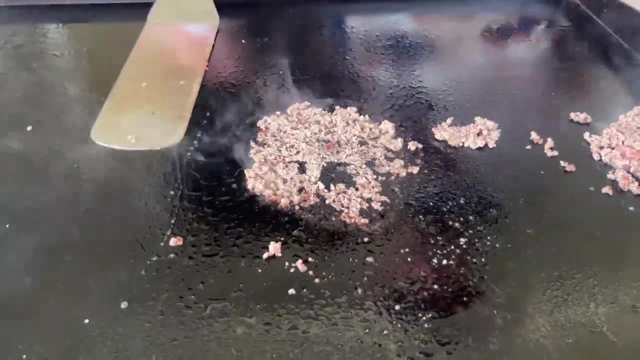 Meaning that you want to get the crust buried down. the griddle story will help you to roll it out. see the difference? okay, we can still get that off the griddle with with correct technique of your spatula. that's why, if you guys will notice in a lot of my videos, we have best griddle spatula. 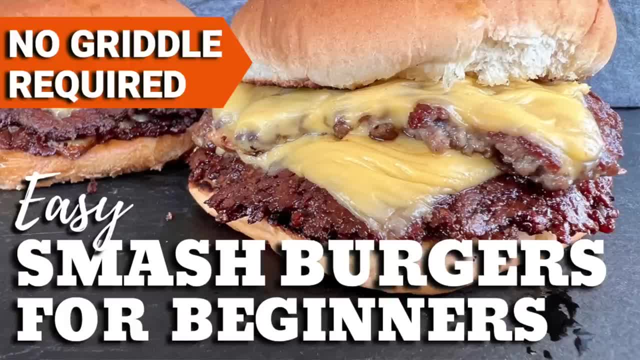 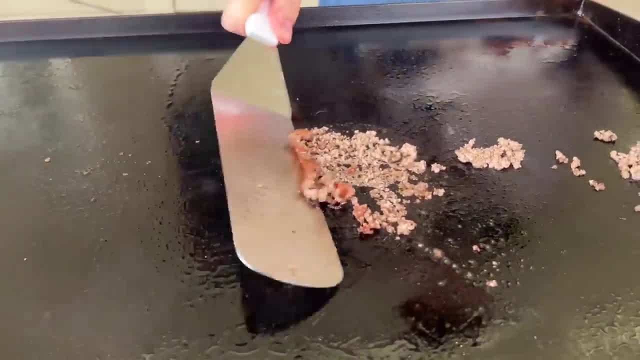 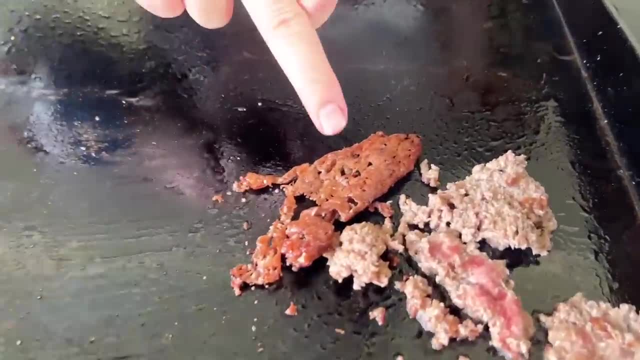 we have the spatulas length. we have everything you need to do to be a better griddler, faster than most. it's because the spatula that you use- okay, see, i'm digging the crust up. now you can see head-to-head the difference in the color. 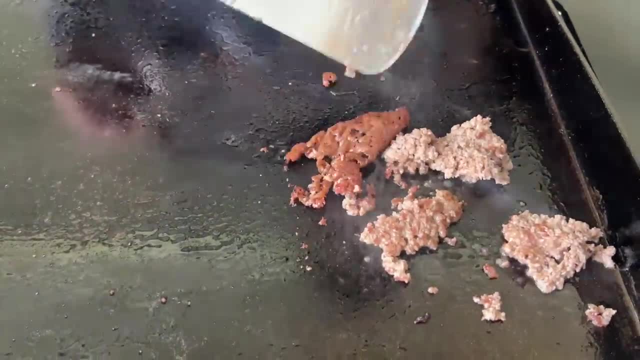 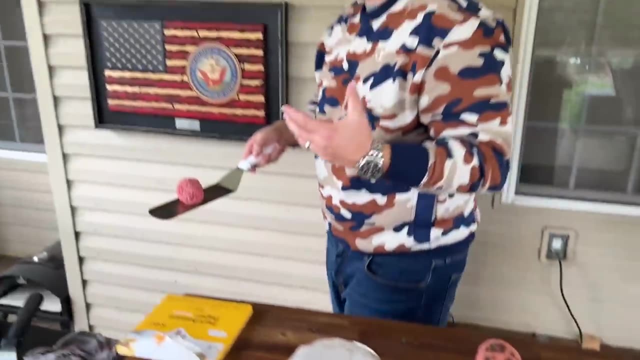 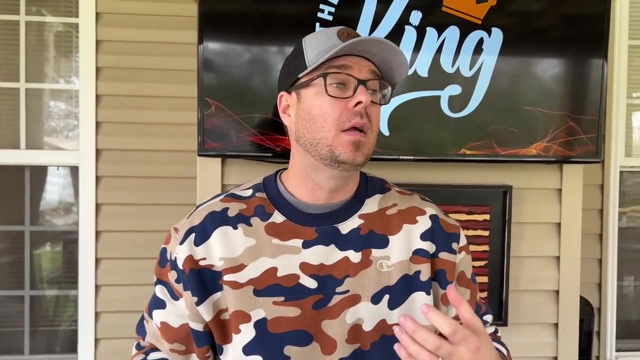 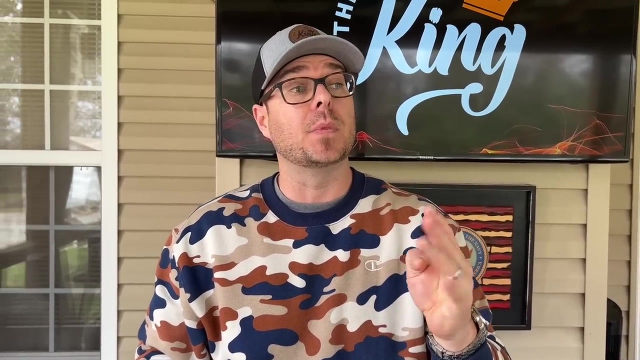 that you look for. okay, that's important. that color is what it's all about. number five on the list over cooking your burger. it's easy to do. we just talked about the difference between having a juicy burger because you smashed it or like like my wife did with her five- um, smash burgers for beginners. We threw my smash burger in the 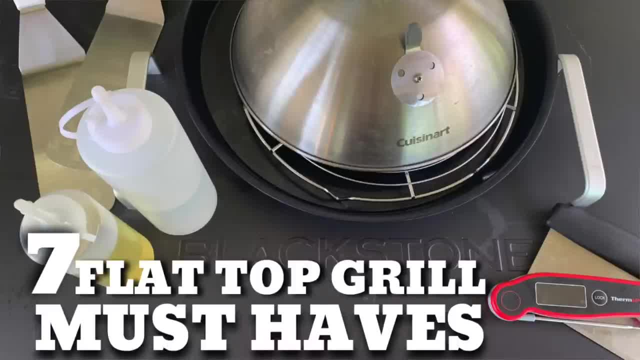 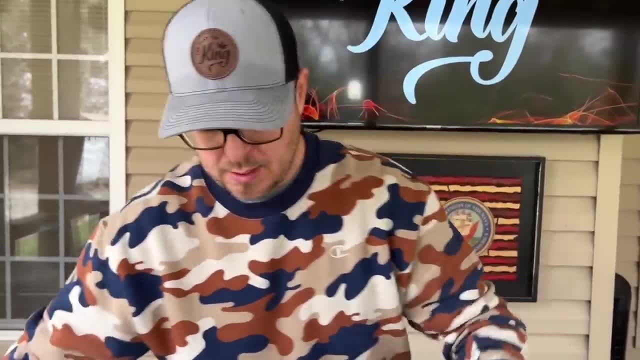 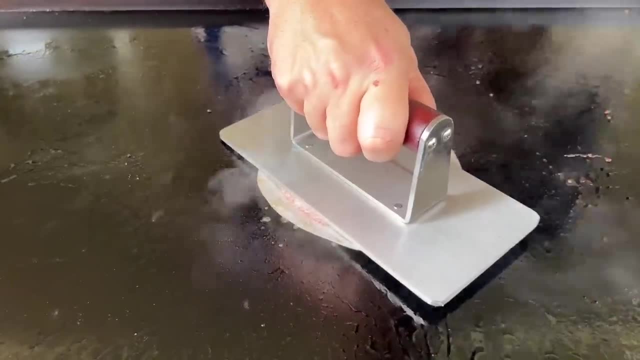 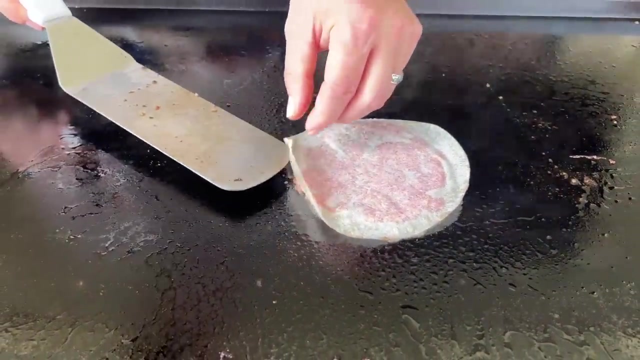 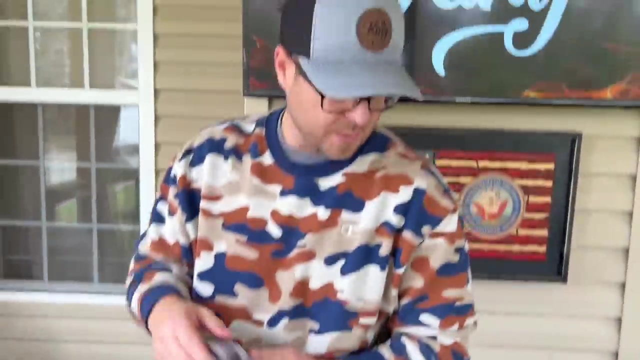 yard. It was way overcooked, Right, But I let her do her thing right. I want to see how she reacts. So we're going to simulate that right now and show you guys what to look for when you're making your smash burger, Why this was going. I would just like to make a public announcement. 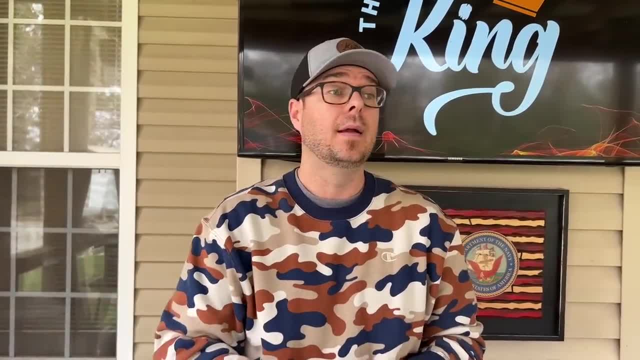 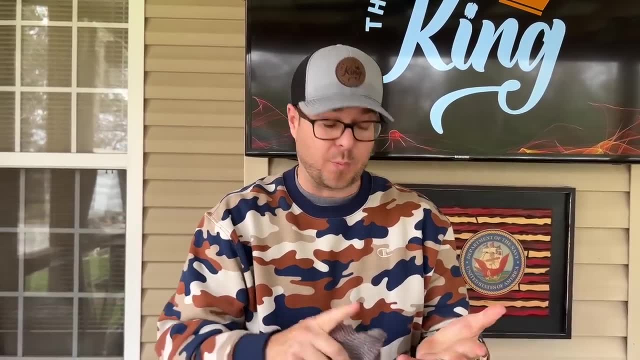 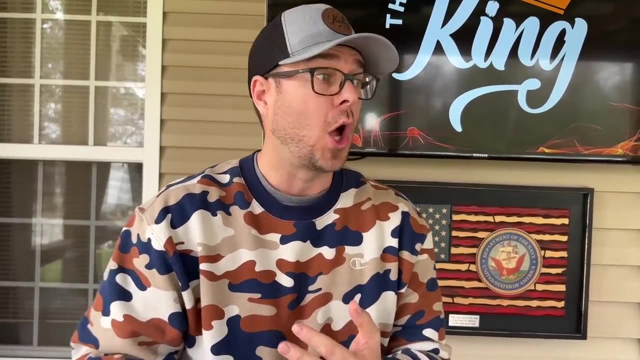 When you're new to the smash burger game or the griddle game, completely Okay, The speed of these things, um, for most people is super fast. You have to have your prep work done. You've got to have a game plan of: if you want your buns toasted, uh, what kind of condiments do you want? Are you feeding? 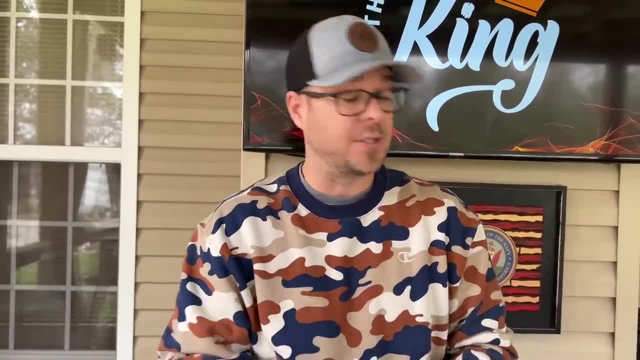 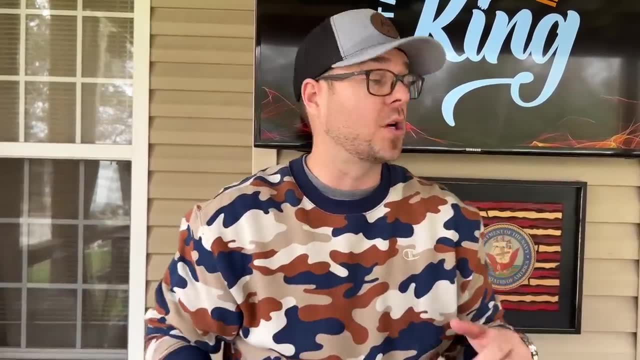 a large group of people. Are you going to have them come through line? There's a lot of things that go into it. A smash burger is thin. You've got a small window to create the greatest burger of all time. Okay, Because the longer it does sit, the longer it's going to dry out like any meat. 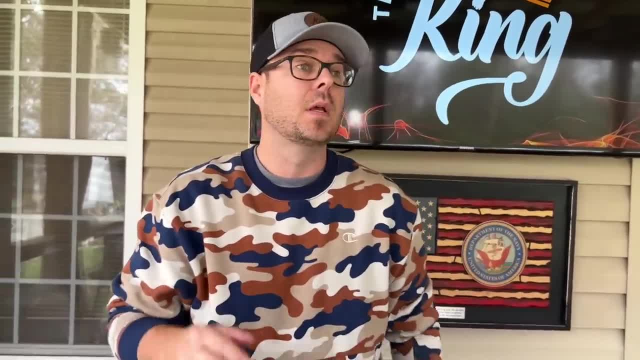 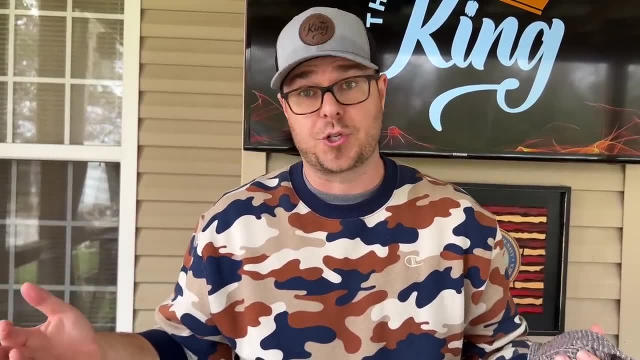 right, But you have a smaller window because your burger is so thin. When you're new to it, don't be scared to come out. Don't don't have 40 people over and expect to make smash burger heaven on your first try. Okay, Once you have your griddle ready and you're 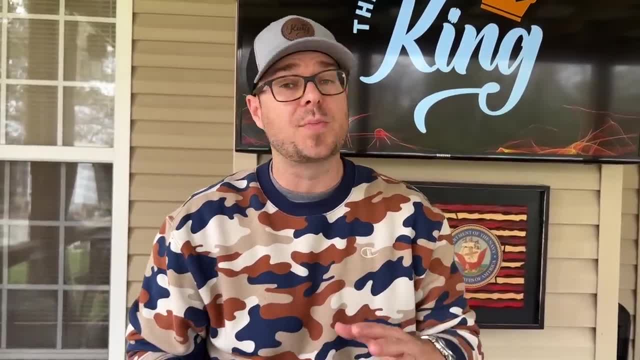 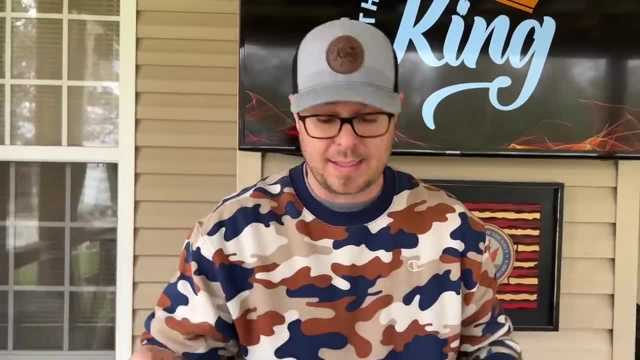 ready yourself. try one burger at a time, not a double smash burger, nothing. You can have it and save it for ground beef. You can do it for spaghetti. You can eat it on the side. We haven't even talked about seasoning. What you want to do is put your burger on there. You want to, naturally. 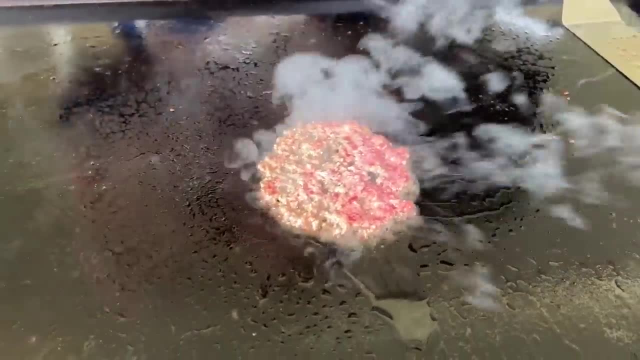 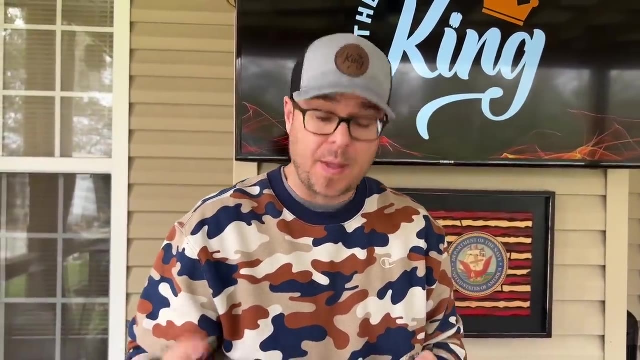 feel what it's like to smash the burger because one that's very important. Once you get that, you're going to know that you're going to be able to eat it. You're going to know that you're going to notice how long it takes, how hard to press, because you'll be amazed how many people just 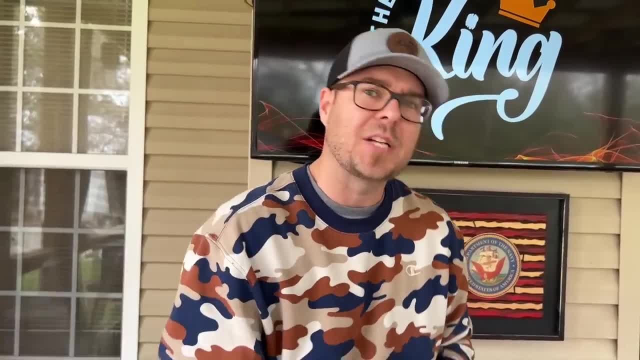 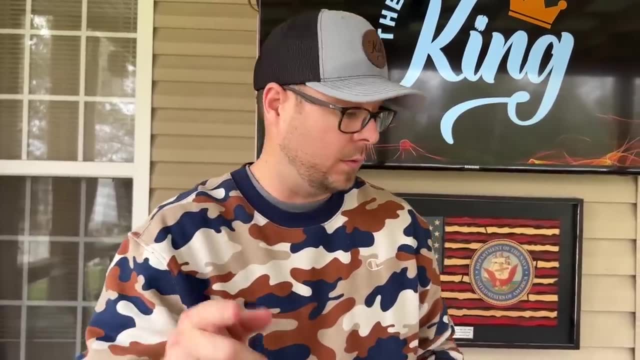 take something and they'll smash it right through the flat top, or they won't smash enough because they're scared that they want. they have a dry burger right. One burger at a time until you feel comfortable. Practice Right. Practice makes perfect. All that has made this burger. 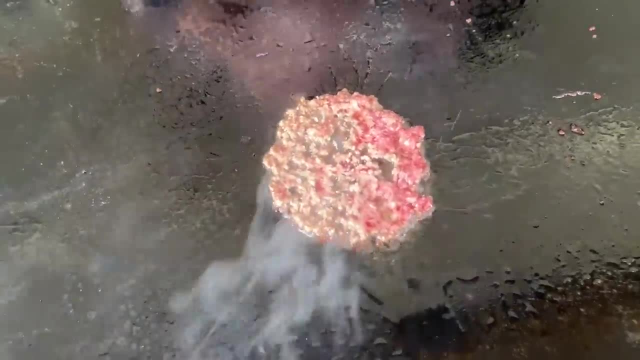 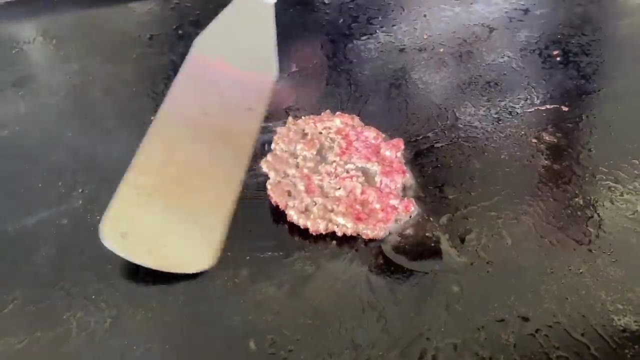 extremely overcooked, which is what happened to my wife, right? Yes, It happens extremely fast, Okay, So we're going to flip it. We're going to get that crust off, right? So let's think about the beginning. The griddle's hot enough. We smash it to our liking. We're getting the crust. 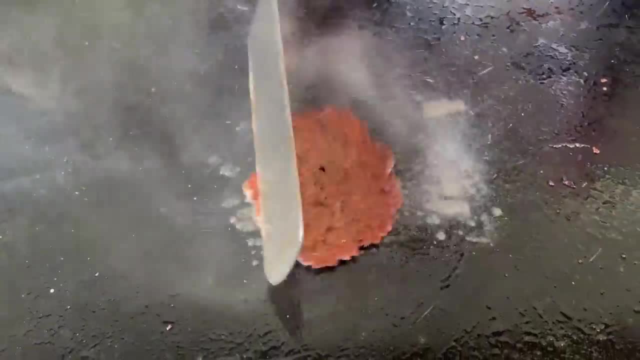 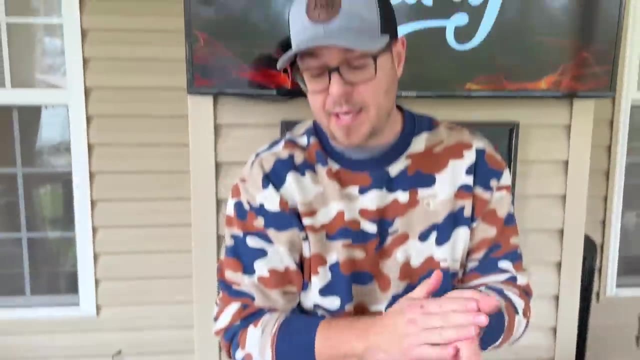 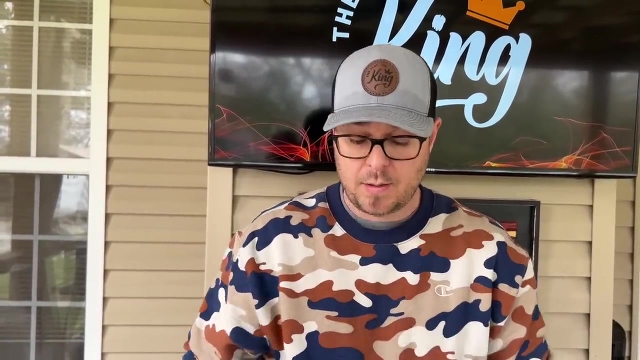 off, but we let it cook too long. Now you're starting to see that crust. right Now you're venturing into the part of an overcooked burger. You've done everything right until this point. You just didn't do it fast enough Flipping it. You didn't flip it fast enough, Right. 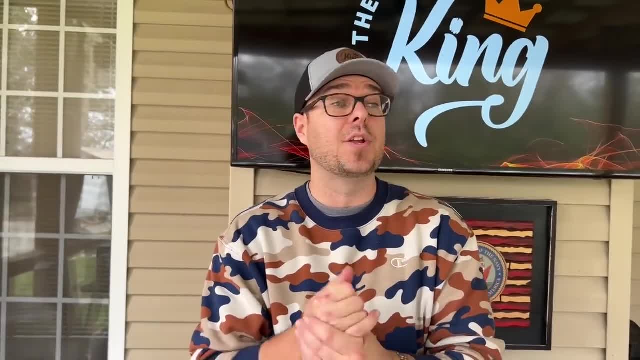 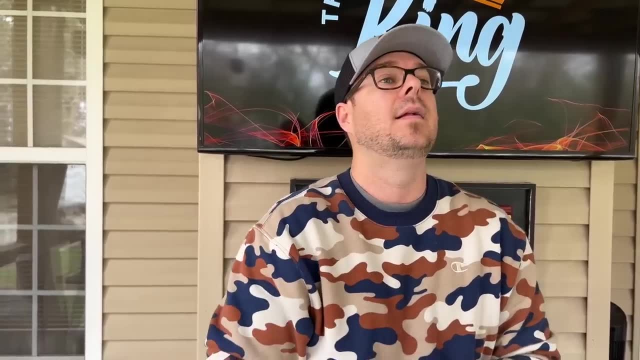 Which is what happened to me, And it was very dry. Most people aren't going to know it. the first time We've got tons of feedback after we did the smash burgers for beginners, especially when you did it. Yeah, That said, thank you so much. 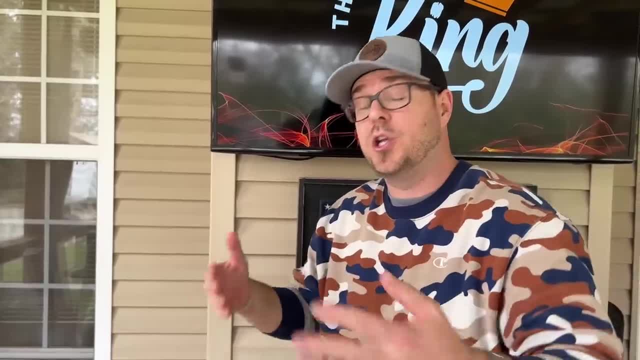 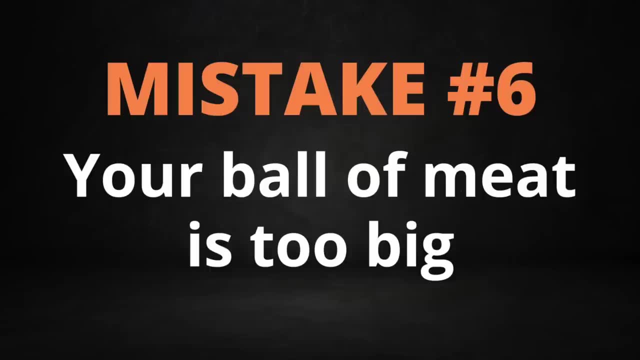 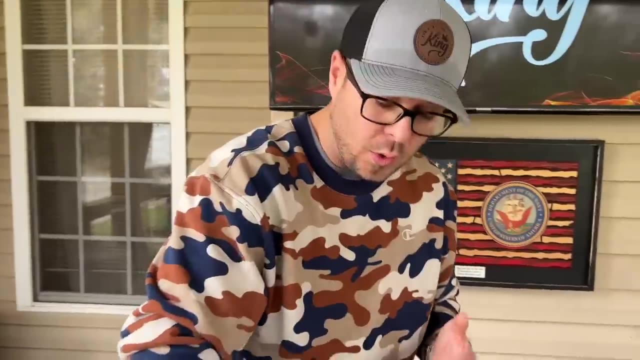 for putting it in a different perspective. Me behind the camera, you here, so we can see what it's like for beginner, And I think that was key to resonate with a lot of people. Number six too large of a patty. I know it's easy to think that like. 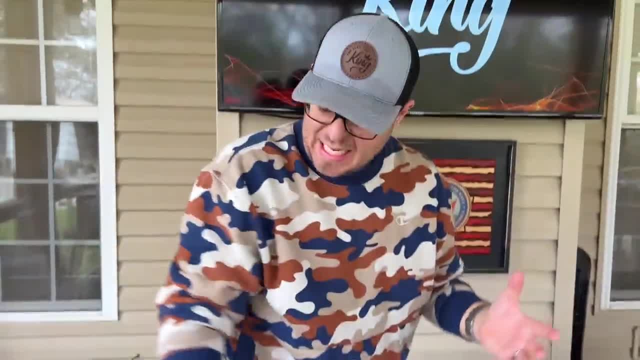 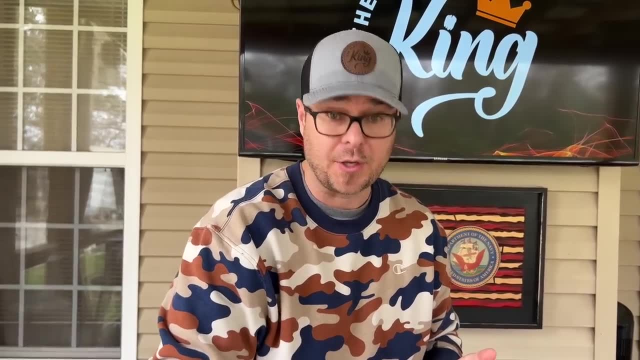 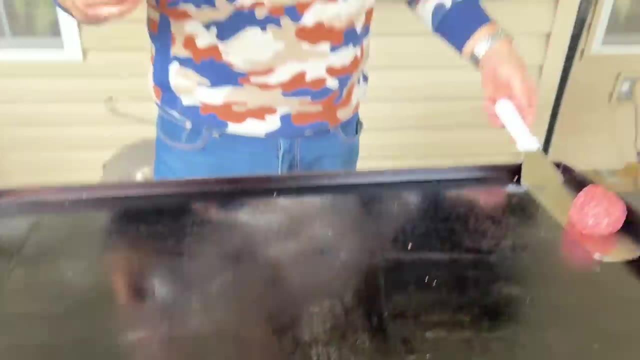 biggest Patty. you want it to be medium juicy, Just like when you season your griddle. you're going to hear it often: Thinner coats of oil are better than thicker coats. Okay, The perfect Patty thickness is thinner than most when it comes to a smash burger. So what you want. 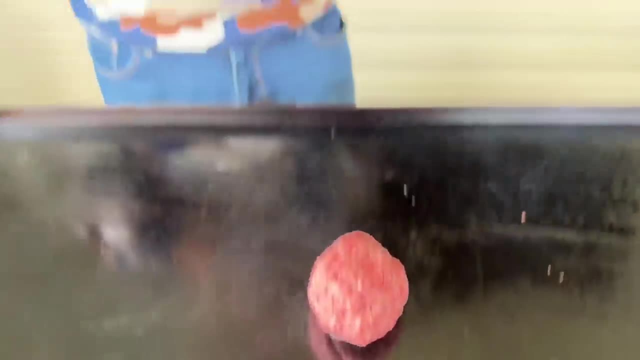 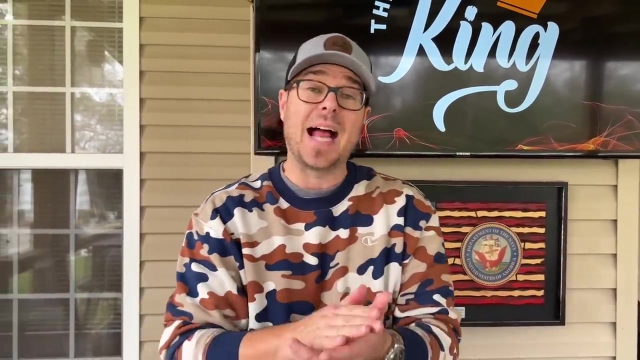 to create is two patties. If you want a bigger Patty or a bigger burger than one Patty, Okay, Two smaller ones versus one big one. To smash it correctly, your burger just gets too big or it's too thick And to do a smash burger. 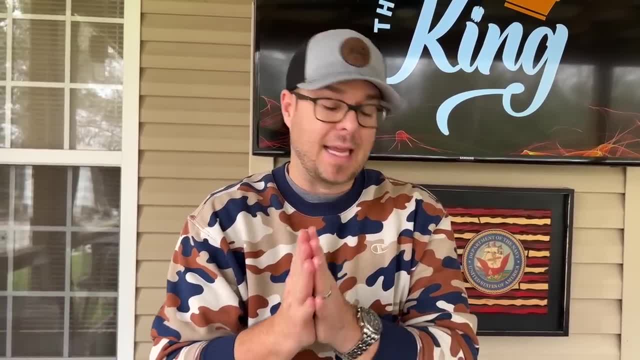 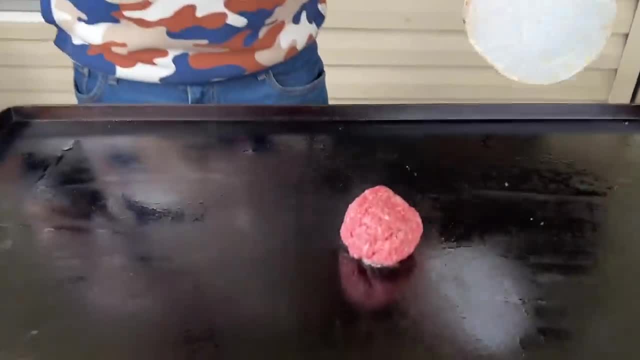 it's not the correct, I wouldn't say correct. It's not the most appetizable Optimal, It's not the optimal, Thank you. So this is too big. Mistake number seven: This is basically two thirds Or six. Mistake six: 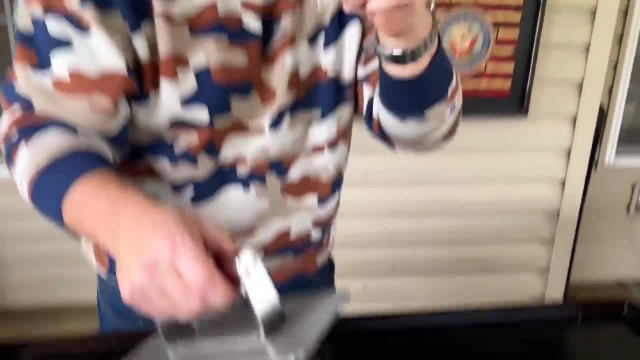 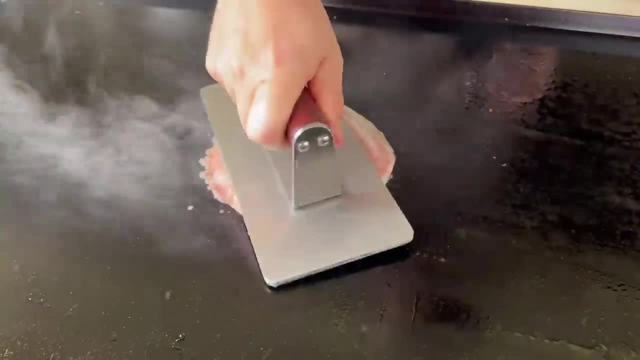 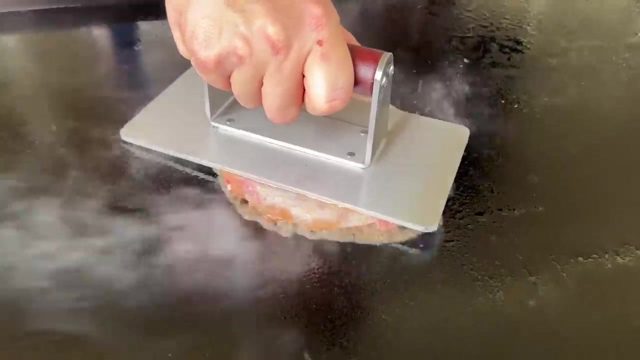 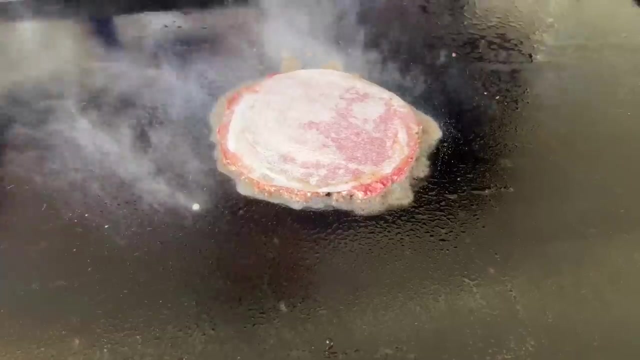 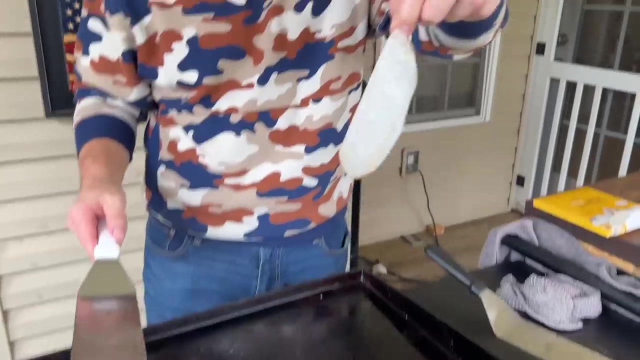 Which one we on Number six, 78.. That's what they feel like. Thanks for staying with me this far. We're going to get a little bit of a. This is a six inch parchment paper round, Okay. This is a six inch parchment paper round, Okay. 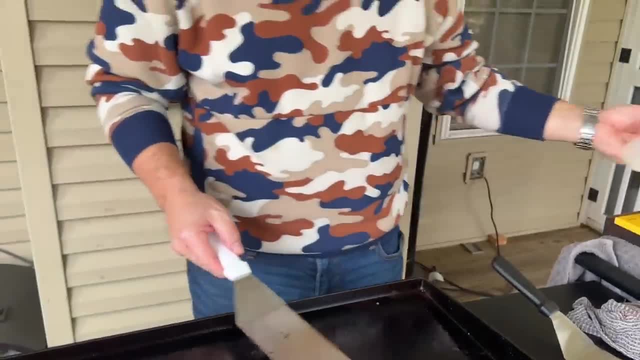 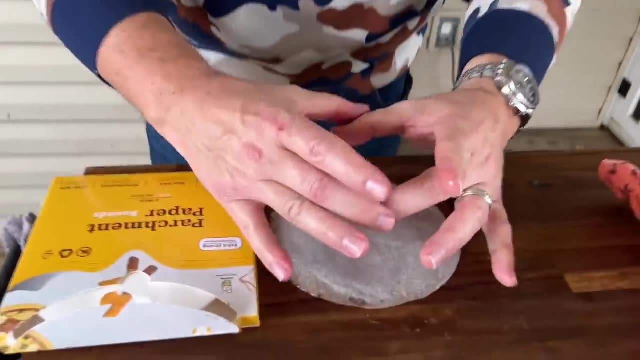 Just to show you, guys, I've been using the same one since we started. If you think of the idea of a standard burger, unless you've got one of those big old burger buns, your burgers is too big. You notice how big that is. 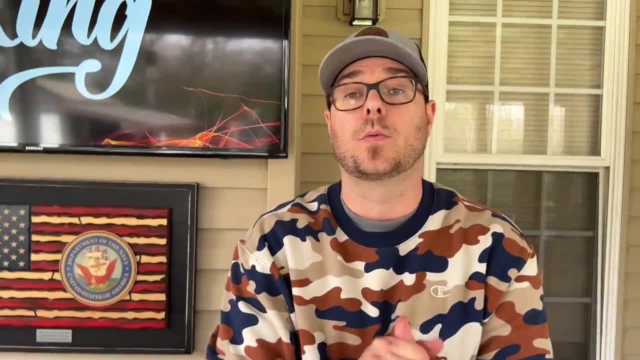 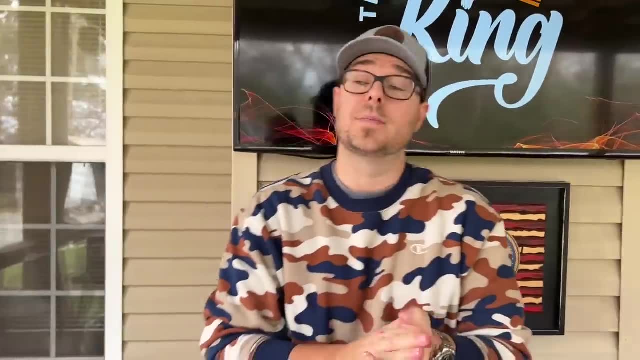 I mean you can't pick that up? I mean everybody would want to, but that's not the realization of the actual burger bun size that you get at the grocery store, right? Do we have a bun to show comparison? No, today I'm doing something old school. 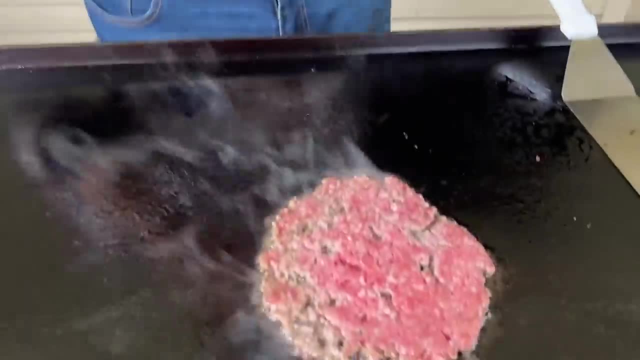 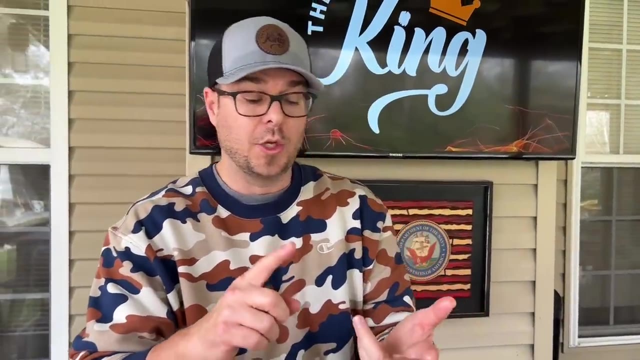 I've been wanting to do it for a long time, so I hope the people that stayed with me this whole time like it. It's a playoff of it. Now your burger can react the same right. You can smash it, you can hold it, you can get it off the griddle and you can flip it faster. 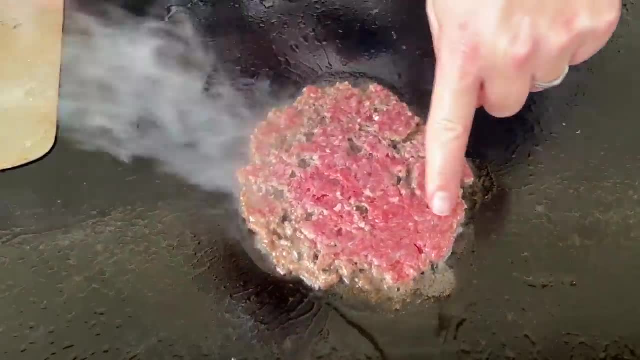 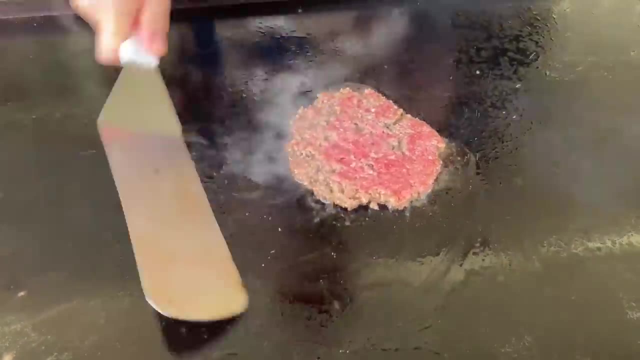 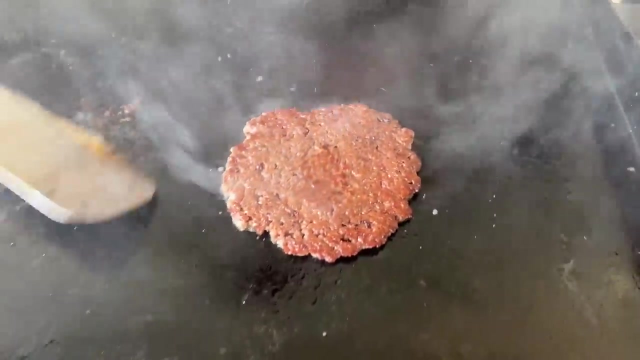 Notice how not everything is completely well done. We've still got some nice medium rare in there, some nice red. That's a telltale sign to flip it right. Notice the lace. That's good, That's a good burger right there. 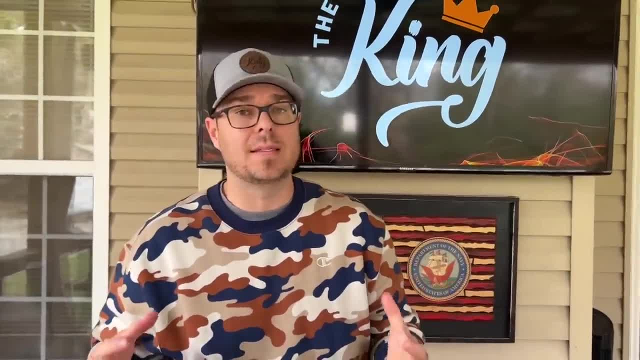 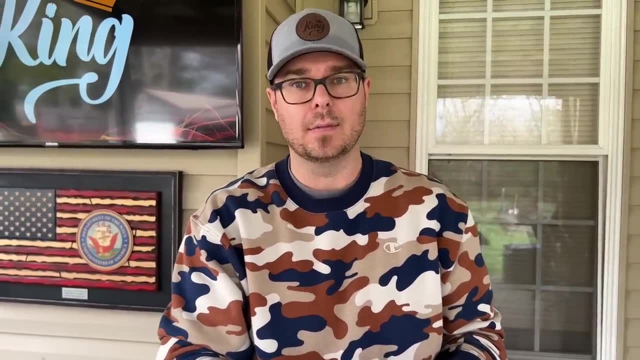 The lace is too big. It's too big. right, There's not a lot, There's not many buns that can hold it. okay, Now that we've talked about all the mistakes that are common, that we see that you could be making, let's make one right, okay? 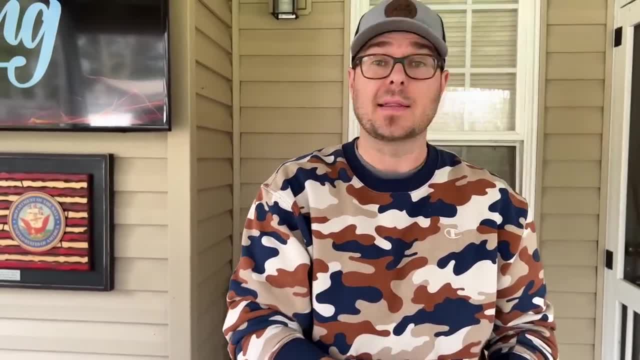 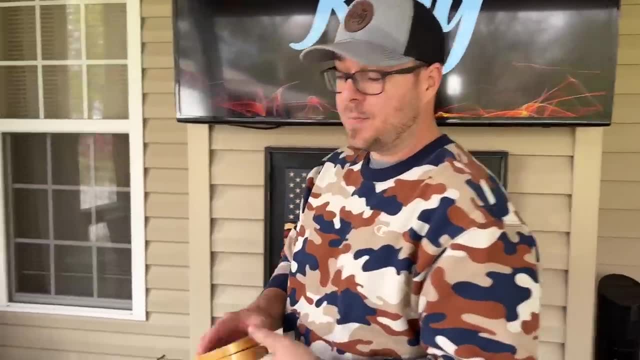 I'm going to throw a little twist in it today, just because I feel like it's about that time for me. We are using white bread When I grew up. let me tell you something. When I grew up, this bad boy was a hot dog bun, a hamburger bun, a sandwich. 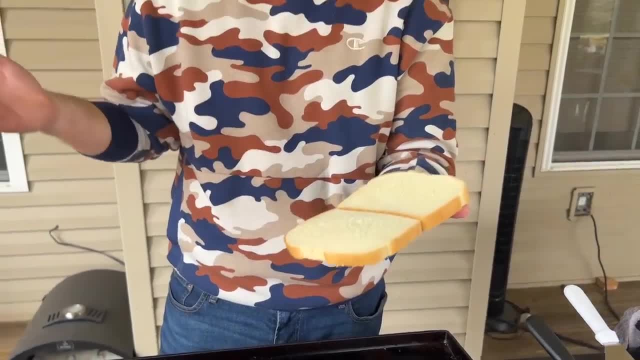 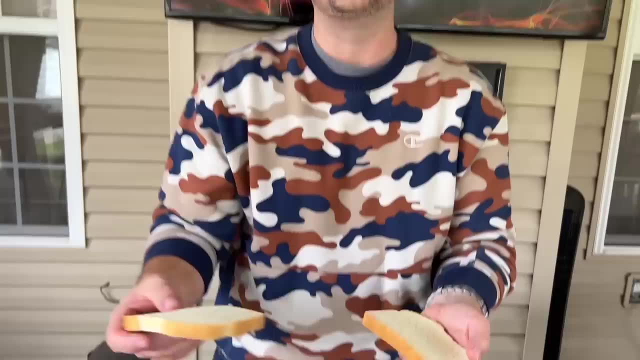 We'd put butter over it and have it with any type of country dinner. That was our dinner roll When my grandmother would make fried chicken. We didn't have anything else like biscuits or anything. Cut this bad boy up. You'd have biscuits and gravy, or we'd call it toast and gravy. 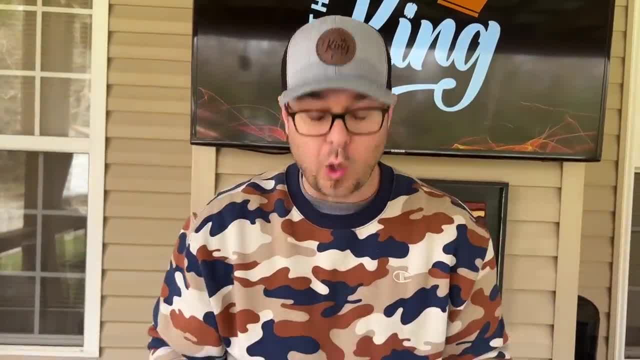 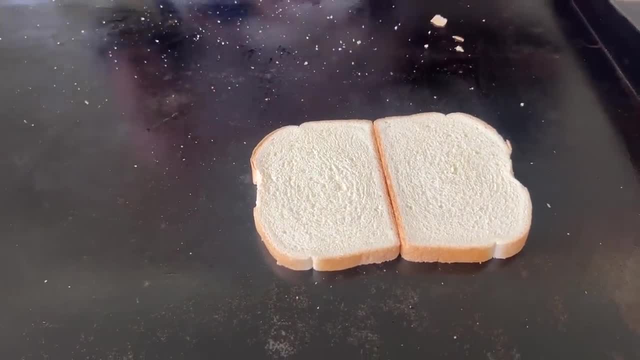 To be honest with you, we didn't even toast it, We just ripped it up. The world's greatest invention: sliced bread. I'm going to put it on the griddle to start toasting, because that's what we're using today. 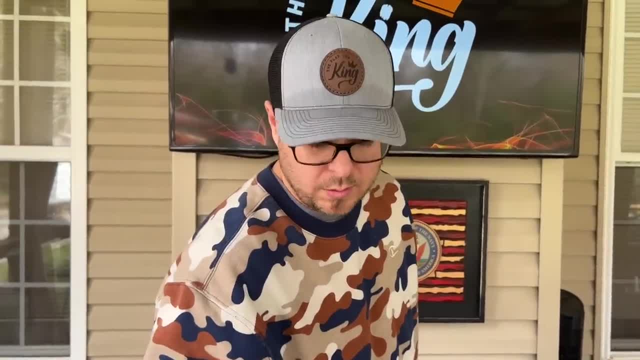 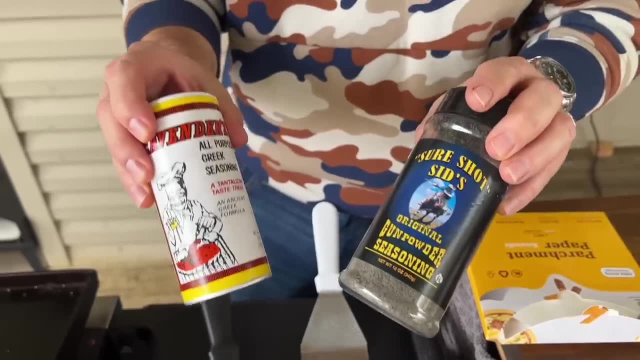 You can use a hamburger bun, of course. Bring it back to old school. We've got our two favorite seasonings. I think this combination on beef right now is probably my go-to. would you say, Yeah, Super good, And we tasted a bunch. 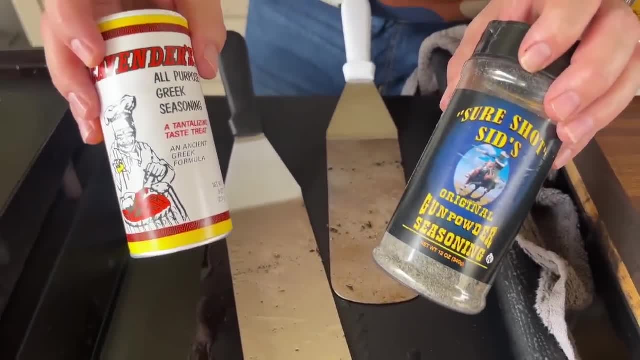 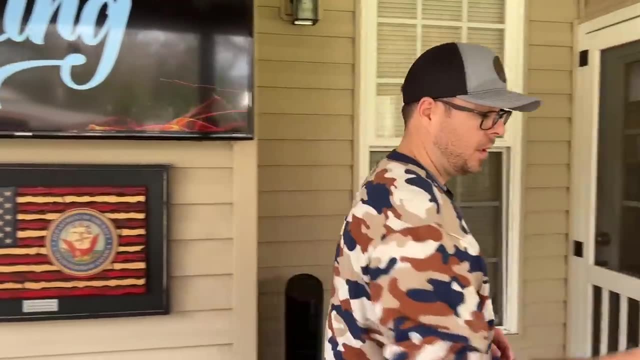 But these two together- and we will have the description and links below- are probably the best combination one-two punch I've found in cooking. Okay, That's one. We've got a little yellow mustard, which there's not much in there. 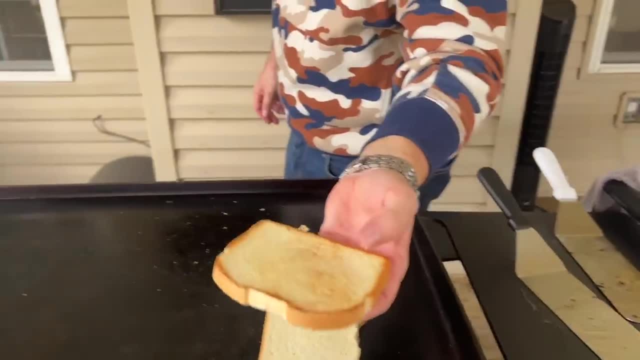 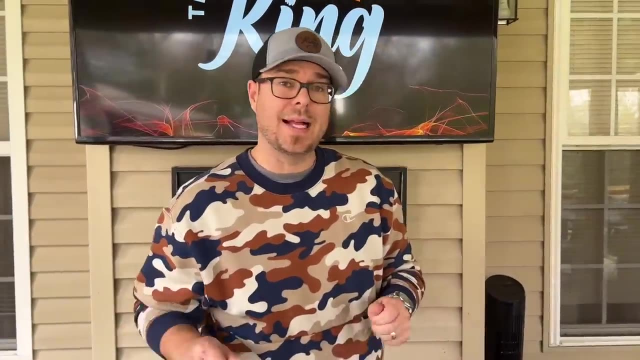 I hope we get some out And a little mayonnaise, Lightly toast in one side. Just move that off the heat, because then the other side we're going to dab in that beef fat that comes off on the flat top. All right, let's go. 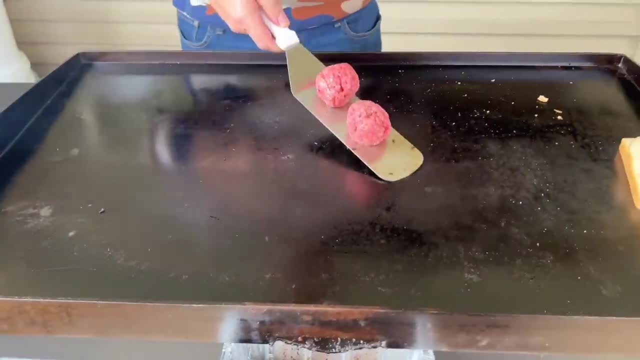 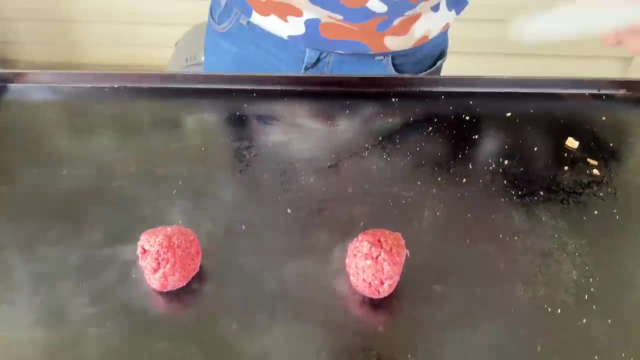 Plenty of space when you smash- okay, You can do that. You've got to remember you're looking at about a six-inch burger. Plenty of space When you're doing your burgers and you're doing multiple burgers at a time. 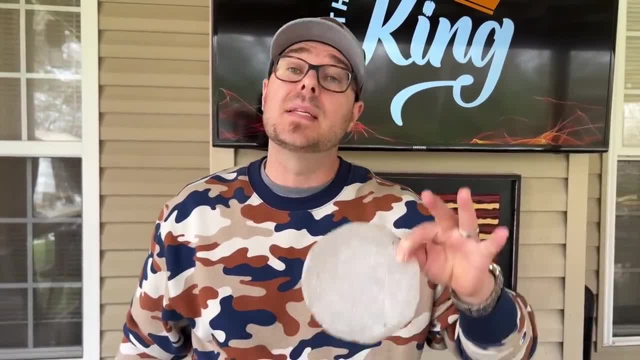 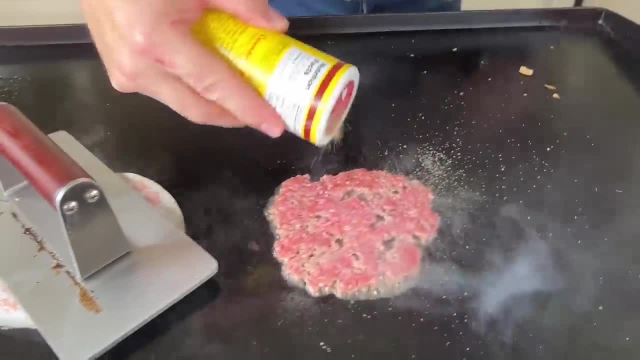 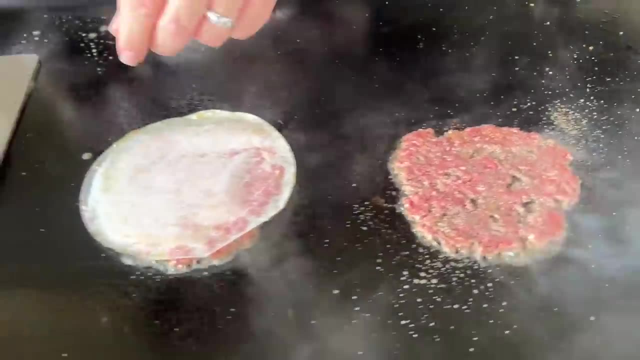 once you get them done, allow your flat top to come back up to temperature. Okay, We talk about that in a ton of videos. Your smash burgers are so thin. typically it only takes one side Of seasoning, Of seasoning, Of seasoning. 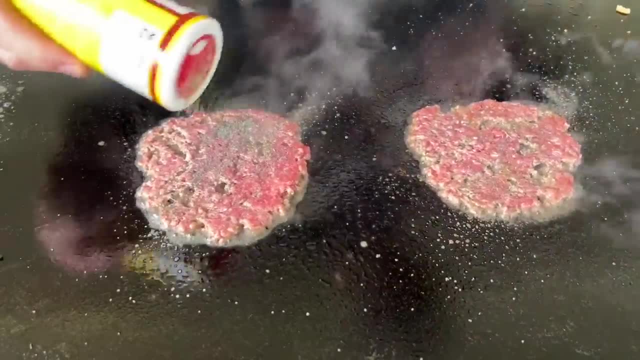 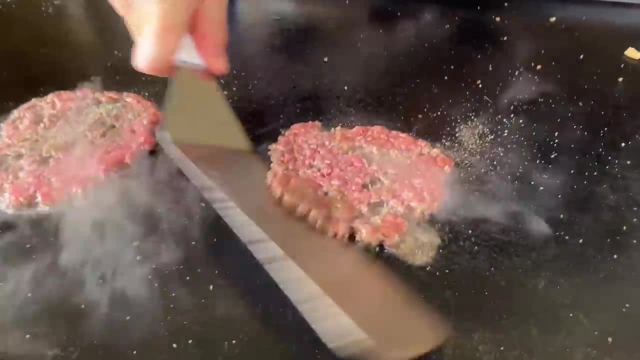 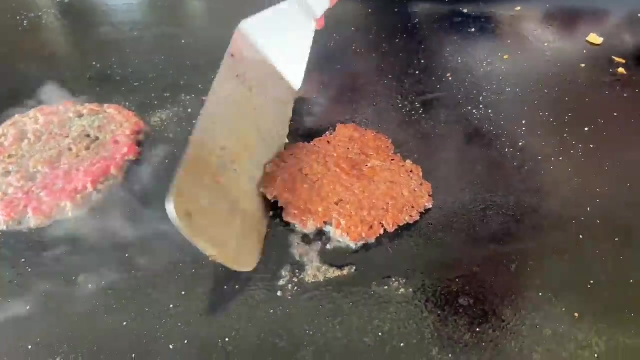 Woo, it's a little too much. We have our cheese ready in hand. We're still medium rare on top. You've got to dig for that crust And there it is All that dark, even color, edge to edge. Same thing over here. 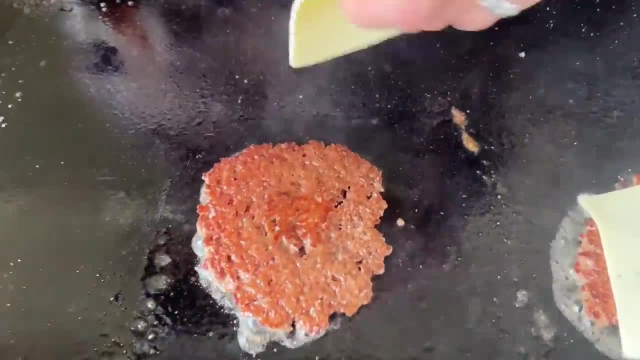 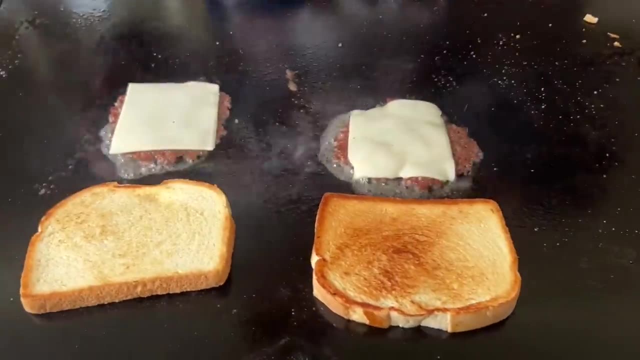 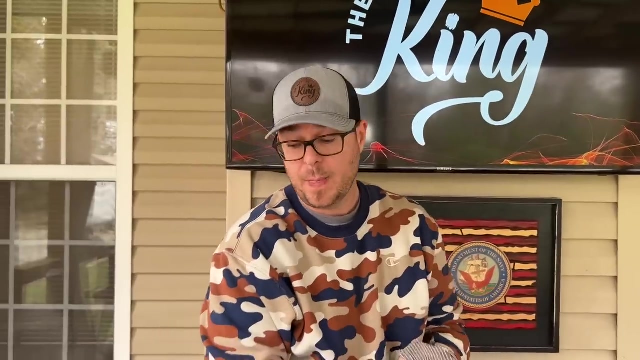 Same thing, Edge to edge coverage, all that browning. Take the other side of those buns, get them toasted in that grease. I will tell you at the speed that I'm comfortable with, to making the best product possible. it would be extremely hard for me on the 36-inch griddle. 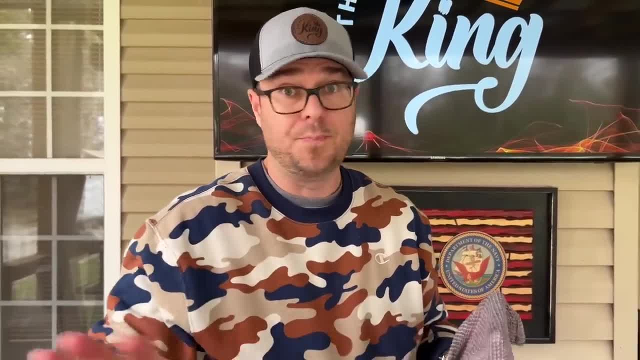 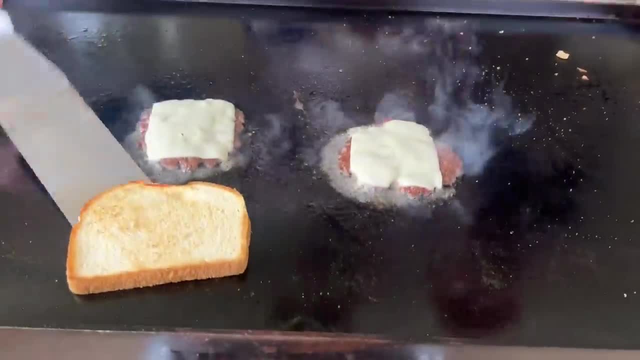 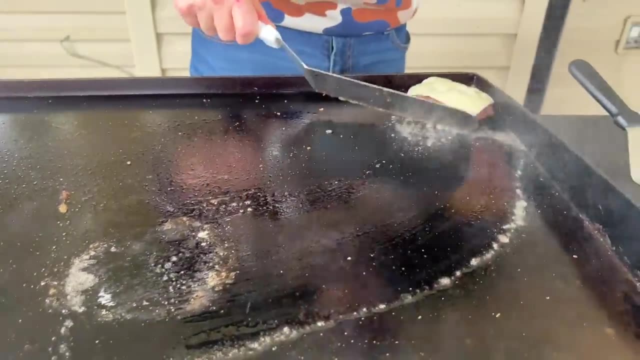 to do more than four smash burgers at a time. The pace of it really happens and you want to be able to create a great burger? okay, Just move it off the side of here. You're going to learn your cool and hot zones. 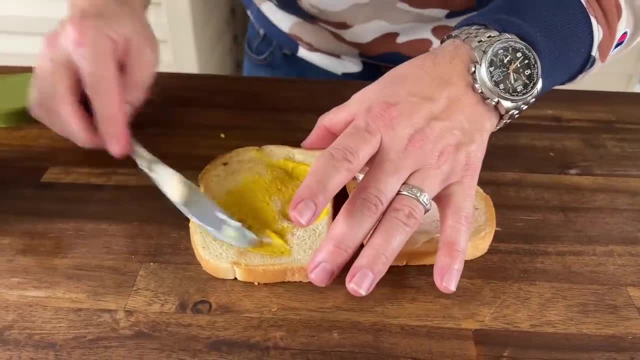 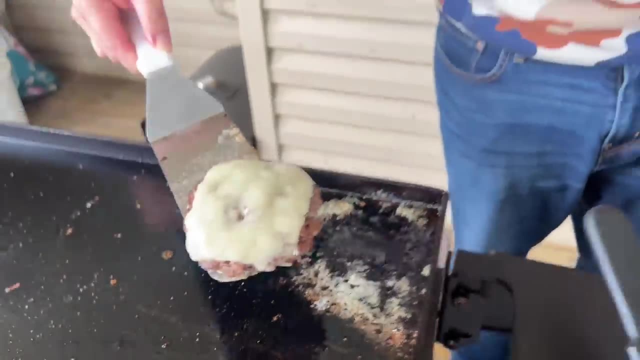 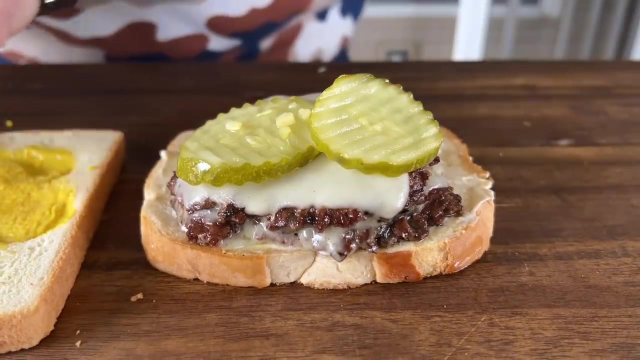 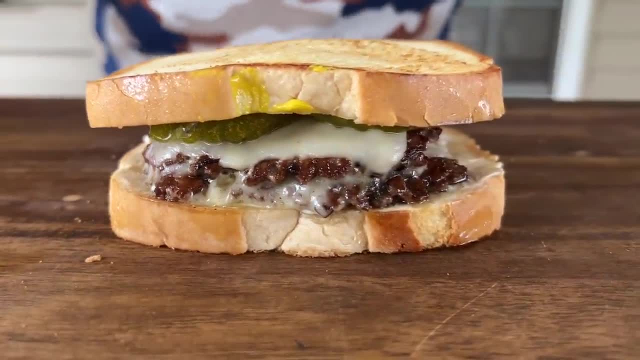 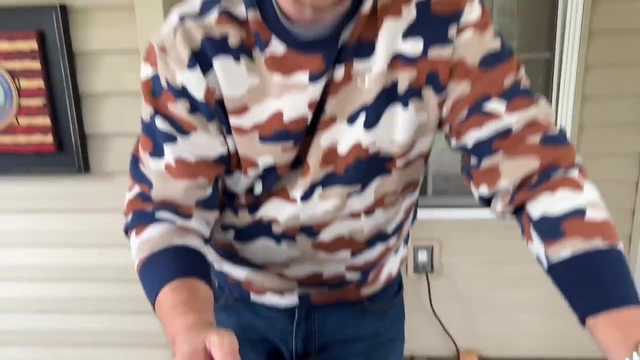 All right, guys, there you go. Super easy, quick. We learned a lot. I've been craving that white bread type of burger because I use what I like, But it's the method behind the madness that helps create the best smash burger.